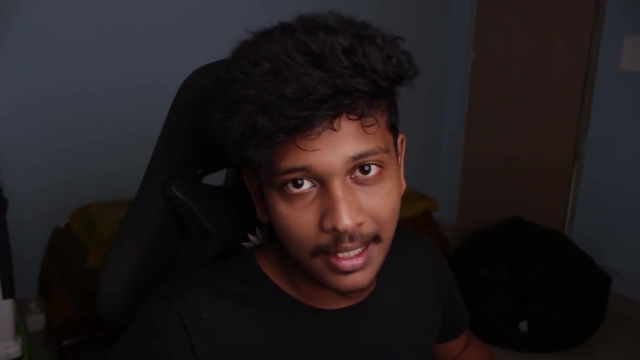 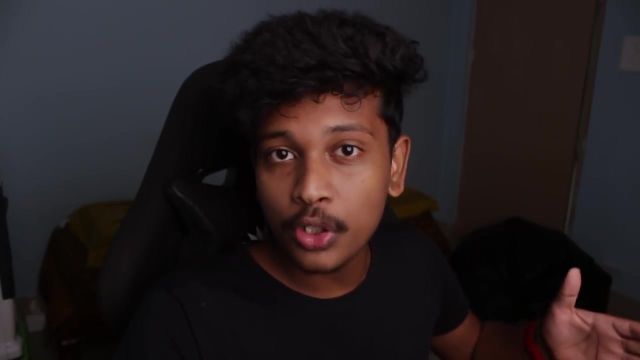 static IP address. It works, even if you're behind a NAT. I know that most of the ISPs, at least here in India, they disable or they do not allow their customers to host web servers from their internet connection. Most ISPs do this unless you subscribe to a business plan. But what I'm going to show you 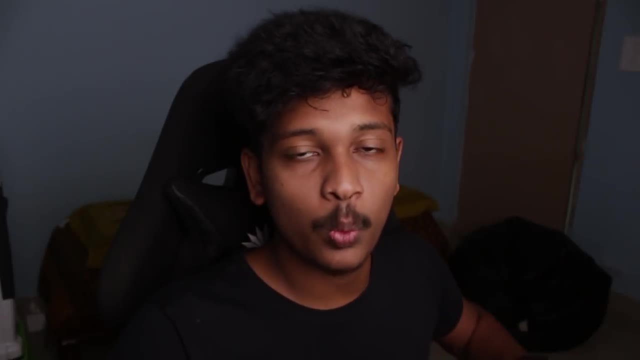 in this video is how to make your website go live from your home computer. So let's get started. This video is going to work for any internet connection, even with a mobile data. You don't need to have a static IP address in order to make this work, So, without further ado, let me show you. 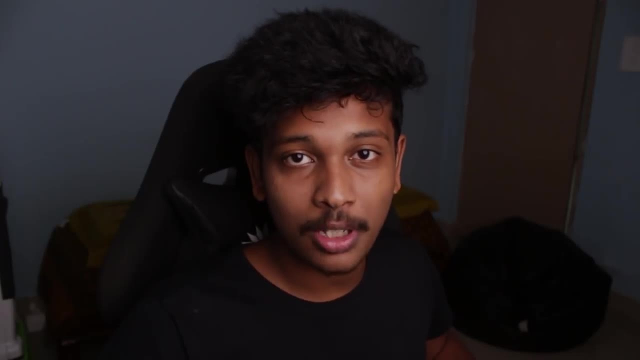 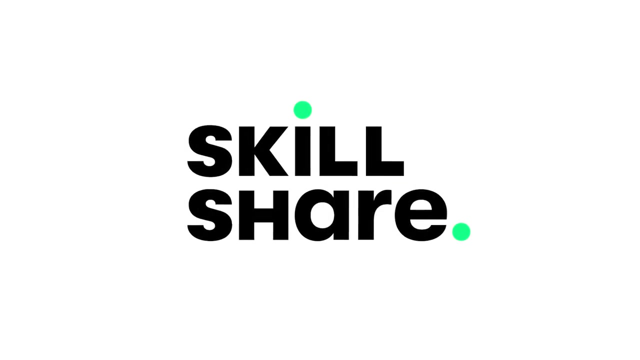 a step-by-step tutorial on how to host a website from your computer at absolutely free of cost. Before getting started, let me take a moment to thank the sponsors of this video. This video is sponsored by Skillshare. Skillshare is an online learning community with thousands of inspiring 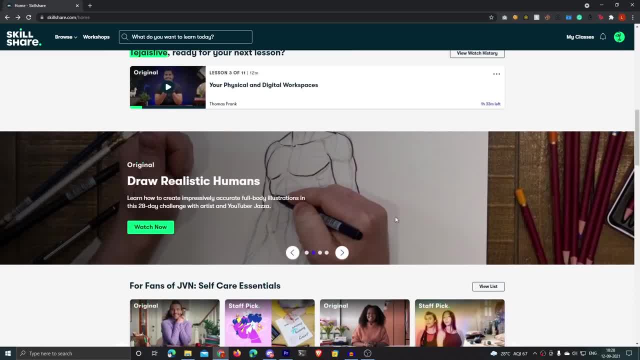 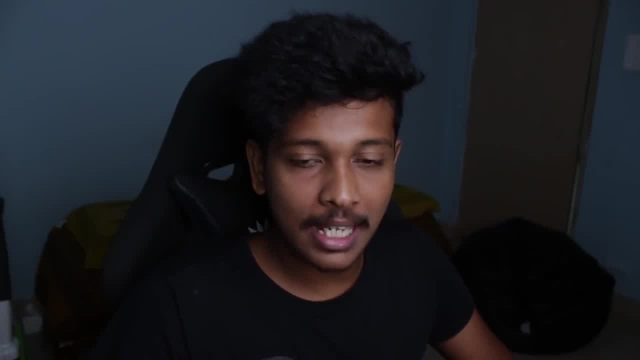 classes for creative and curious people, Explore new skills, develop existing interests and get lost in the world of online learning. If you want to learn more about online learning, go to wwwskillsharecom. I've been using Skillshare for a while now and I must say that it is one of. 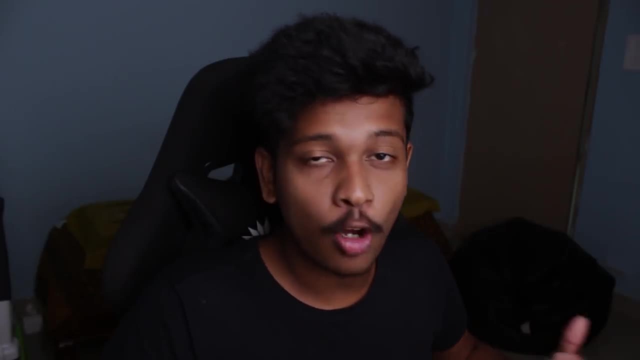 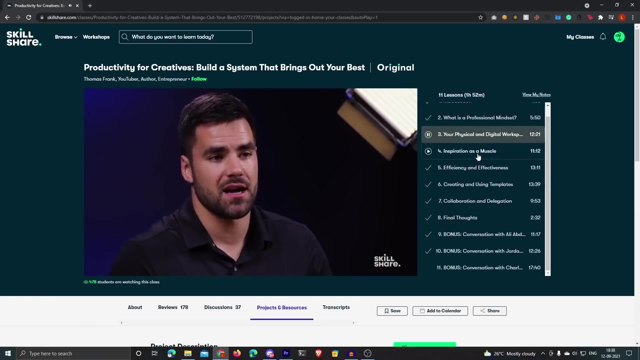 the best platforms available out there to learn new things and follow your passion. For example, I've been taking this class called Productivity for Creatives by Thomas Frank and I must say I really found it very informative and useful And it really helped me to better organize my 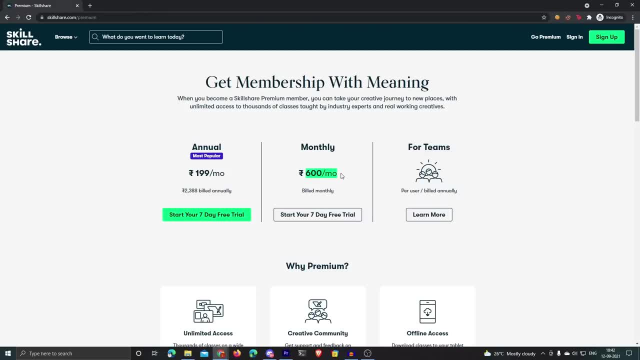 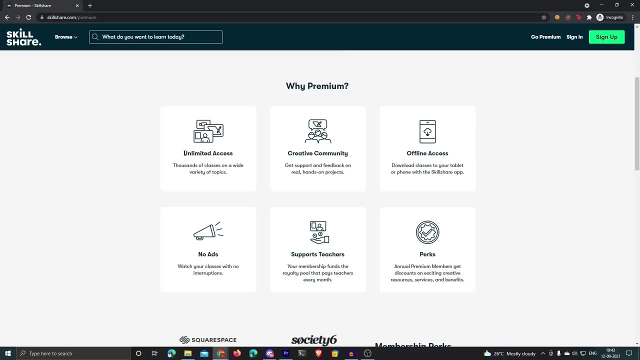 workflow and to be more productive. The thing I like about Skillshare the most is that you can watch unlimited classes for just $10 a month, and that, too, without any ads. You can also join Skillshare live classes to experience real-time inspiration as you connect with popular teachers around the world. Skillshare is always launching. 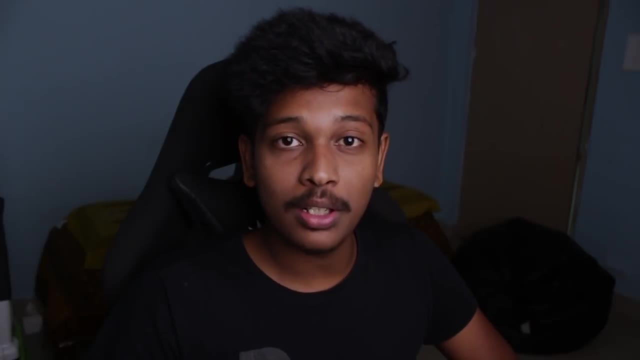 new classes. so if you're interested in something but you don't know where to learn it from, then make sure you check out Skillshare and you will most probably find the skill that you're looking for on Skillshare- And here's the good news- The first thousand of my subscribers to 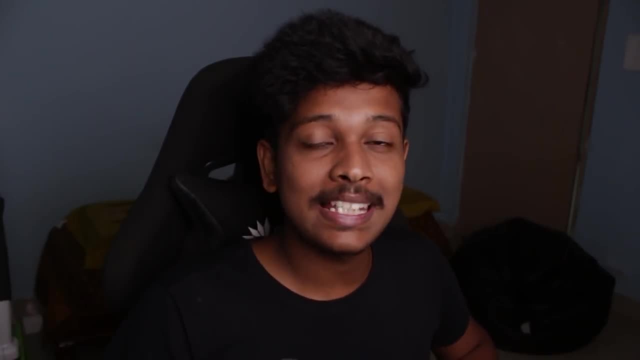 use the link in the description below will get to use Skillshare Premium for free, for free, for free for one whole month. So what are you waiting for? Hurry up and use the link in the description below to sign up for Skillshare and get one month of Skillshare Premium for absolutely free of cost. 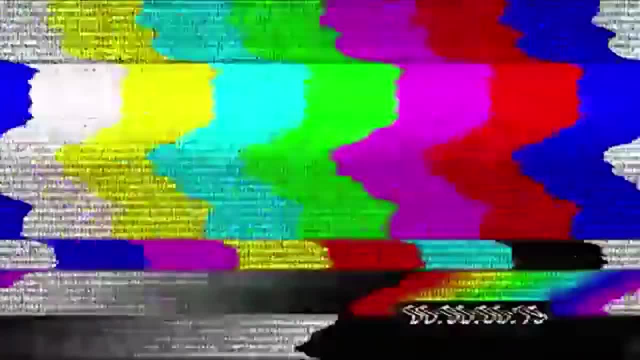 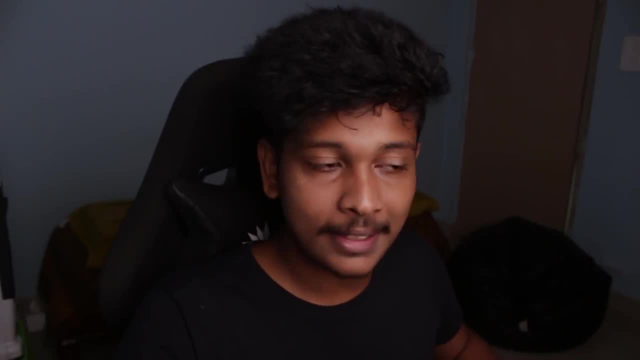 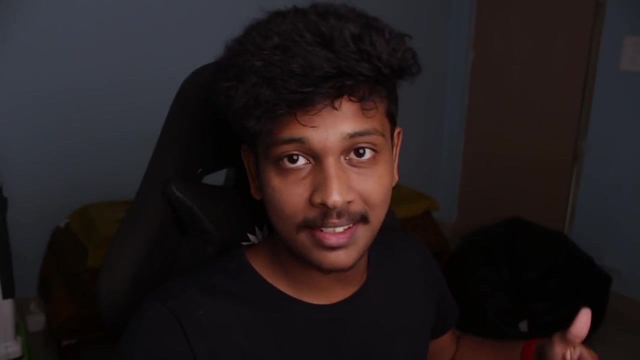 So go ahead, start exploring your creativity today. So the first thing you need is a web server, which is basically a software you have to install on your computer so that it can host, or in other words, it can serve the website that you want to host whenever someone sends it a request. There aren't many. 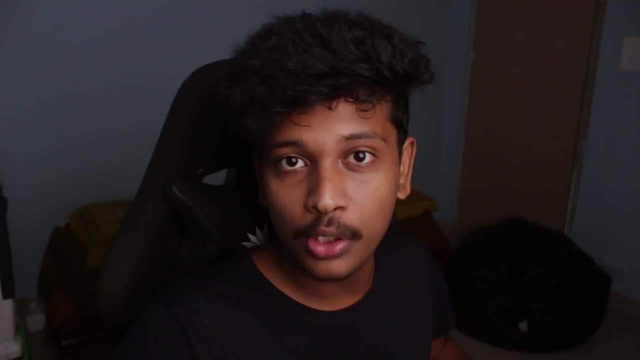 apps available, and one of the most popular ones is Apache, and we are going to use Apache in this video. You also need a database management system because we are going to use WordPress to actually create a website and host it, So we'll be using MySQL as the database management system. 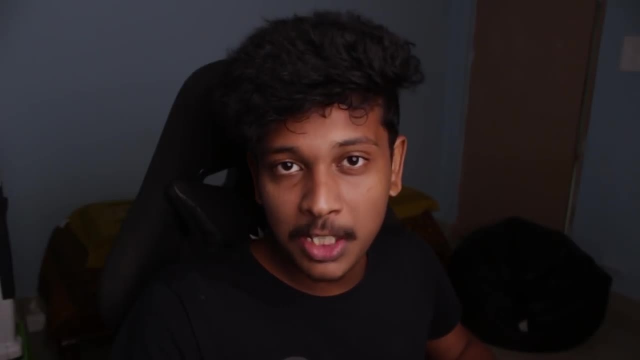 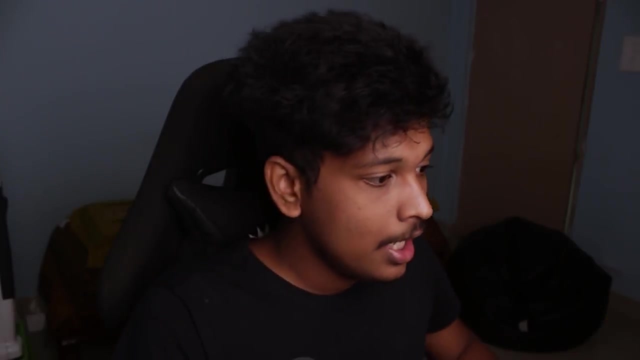 and in order to install these two, the web server and the database management system, you could just install XAMPP. XAMPP is basically a PHP development environment, which means it basically comes bundled with all the required tools in order to, you know, develop and publish a website. basically. 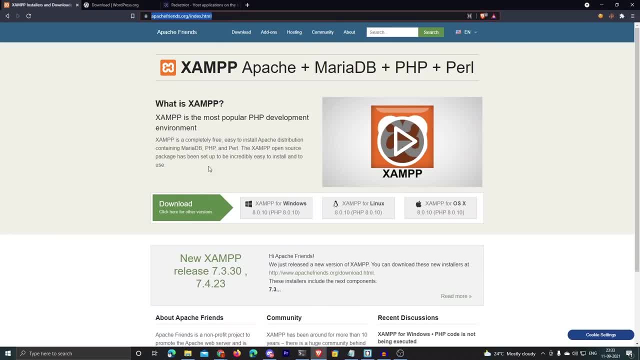 So you can go to apachefriendsorg and you can download XAMPP. It is available for Windows, Linux and OS X And, in case if you did not notice yet, I am going to do this in Windows, so I'm going to download XAMPP for Windows. So before doing that, I would just like 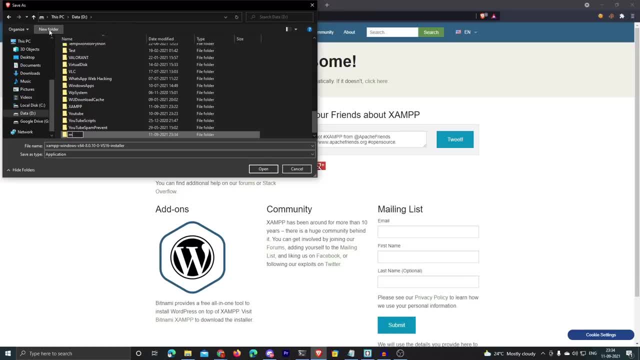 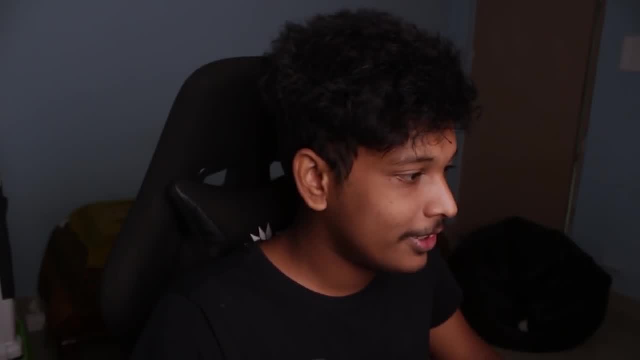 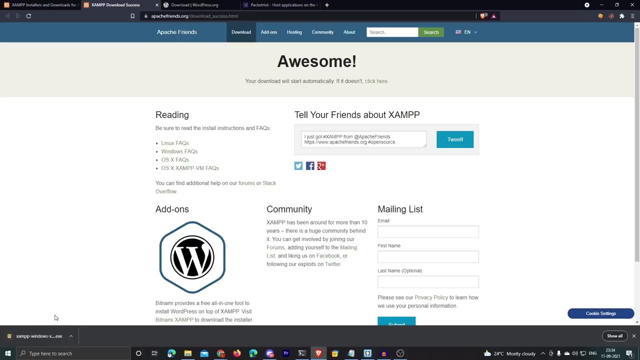 to create a new folder and I'm going to name this as My Awesome Website. That's a lame name, but it works for just the demonstration. So I'm just going to save all the files inside this folder, just to keep it organized. So I have downloaded XAMPP. Once it's downloaded, I'll just 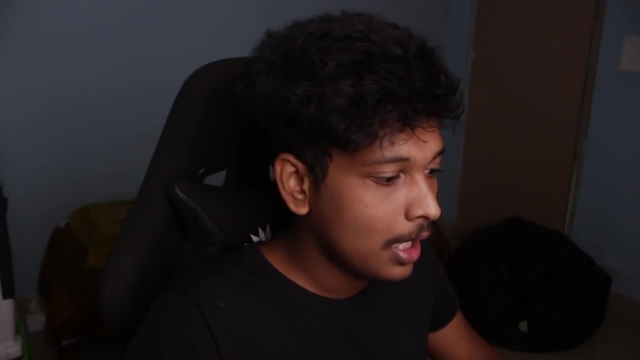 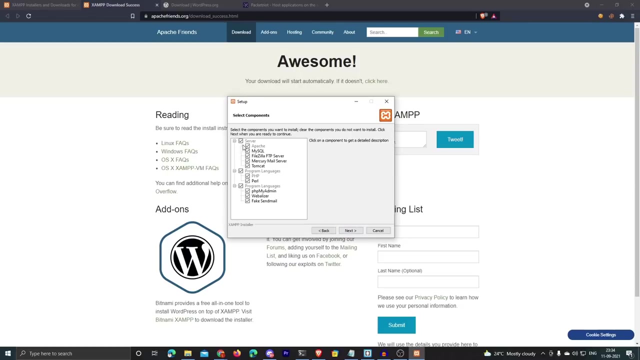 open it and that should bring up the installation wizard for XAMPP. There you go. That's the installation wizard. Click on next and you don't have to change anything in the screen. Just click on next. So in this screen you choose the installation directory of XAMPP By default. 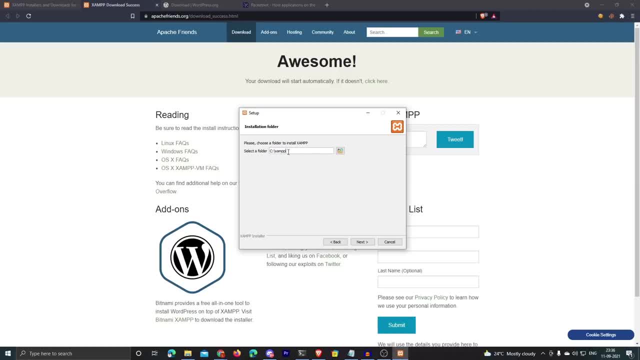 it's going to install in your C drive. Now you can change the installation directory of XAMPP. You can change this if you wish, but it is actually essential that you remember the directory where XAMPP is installed, because we will be needing it for other steps in this tutorial. 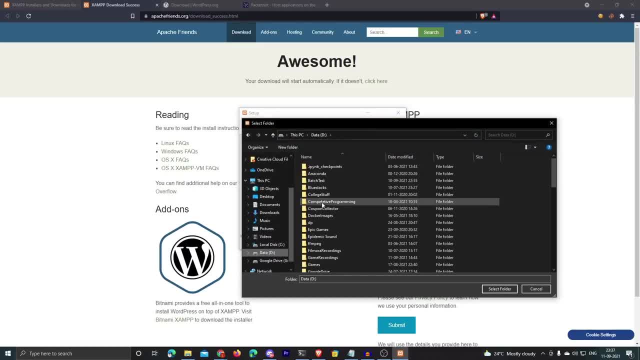 So I am going to change my installation directory to my D drive. You don't have to do this, but it's just a personal choice. I would like to keep my XAMPP in my D drive in a folder called XAMPP, So 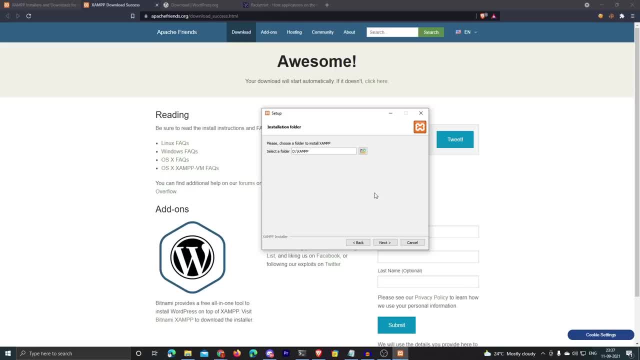 I'm going to set the directory as D//XAMPP. Click on next, again, next, again, next, and that is going to install XAMPP in my D drive. So I'm going to click on next, again, next, again, next, and that is going to install. 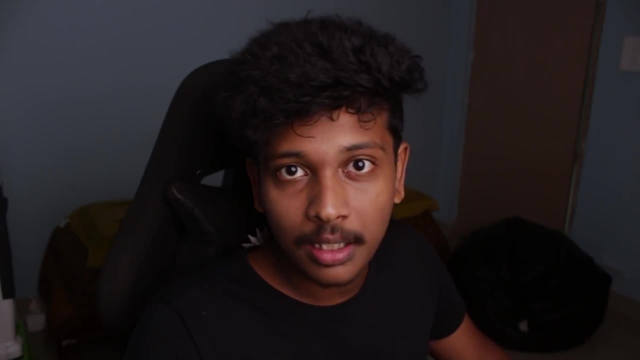 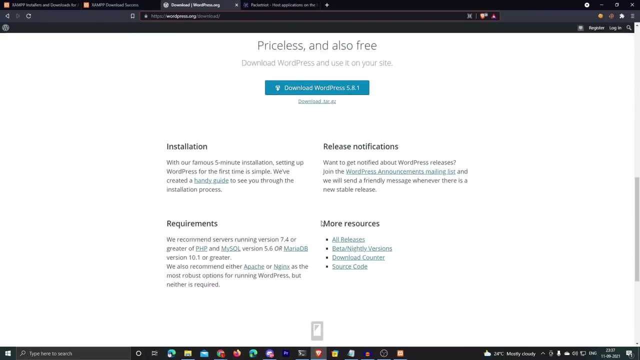 XAMPP on our computer. Now, it's going to take a while for XAMPP to be installed And meanwhile what you can do is you can go to wordpressorg download and you can download WordPress source code. Now, as I already said, we are going to use WordPress to create a website. If you don't know, 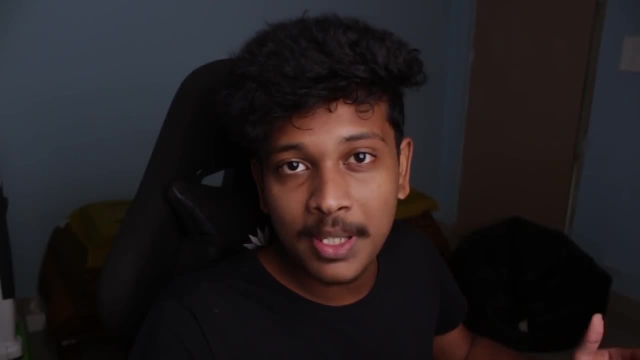 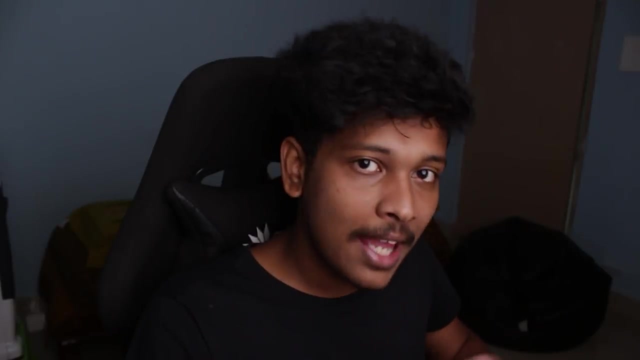 what WordPress is. it is basically a content management system using which you can build a website or a blog. You don't have to write code in order to build a website using WordPress. Of course, you can write code if you want to customize it, and you can do whatever you like Once you install. 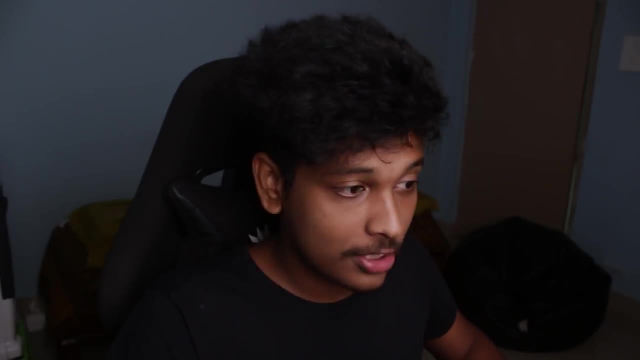 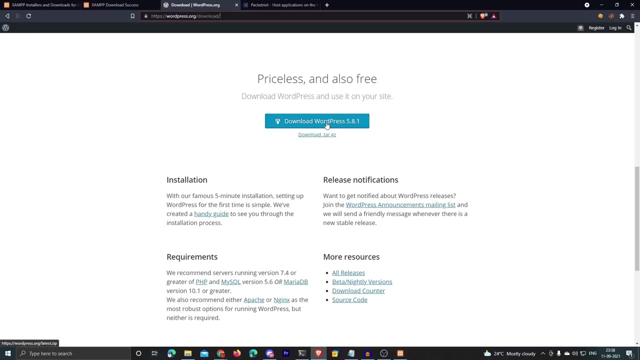 WordPress. you can go to your admin dashboard and customize your site as you want. You don't have to write any code. So I'm going to click on download WordPress. Make sure you download the latest version of WordPress, which in my case, as of making this video, is 5.8.1.. So if I click, 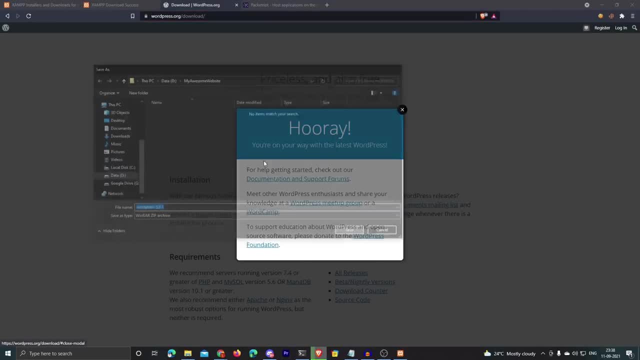 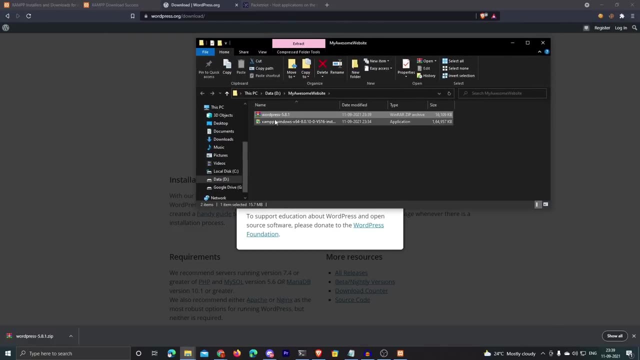 download. it's going to download and I'm going to download it to my, to the same, my awesome website folder, And I will just go to the downloads and there you go. You can see that this is a zip archive, so you will have to unzip it. You can make use of any unzipping utility, like 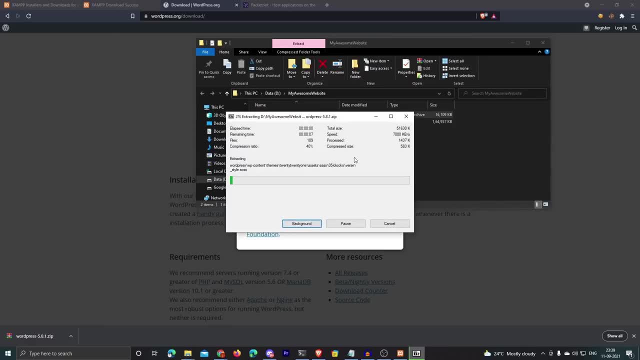 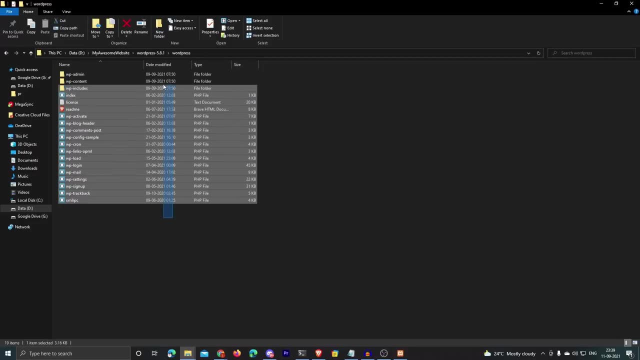 WinZip or 7zip. I'm going to extract it with 7zip. There you go, The extraction is done and you can see these are all the source code files of WordPress. Now we need these files in order to install WordPress on our Apache server. So meanwhile, let's look at how XAMPP is doing in. 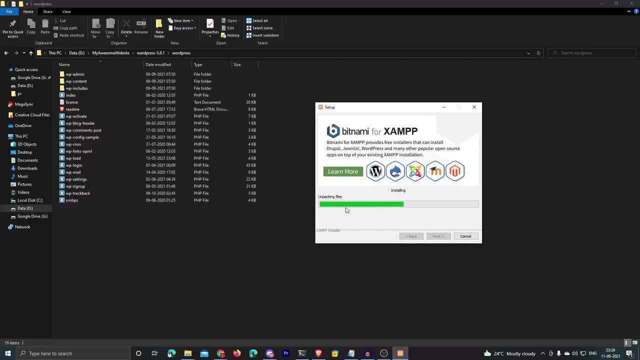 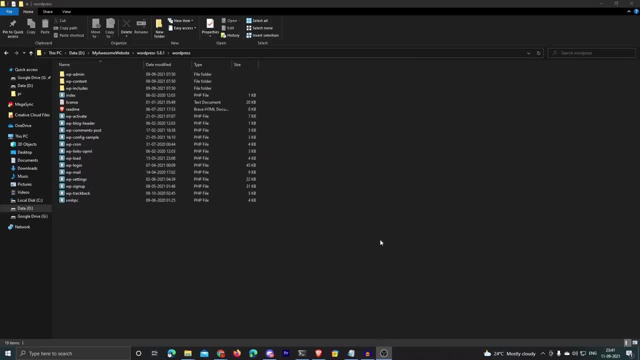 the background. So it is almost done, halfway done, actually. So, yep, Just be patient and wait for XAMPP. So there you go. It seems like XAMPP has finished installing. If you click on finish, that should automatically bring up the XAMPP control panel, which looks like this: Now you 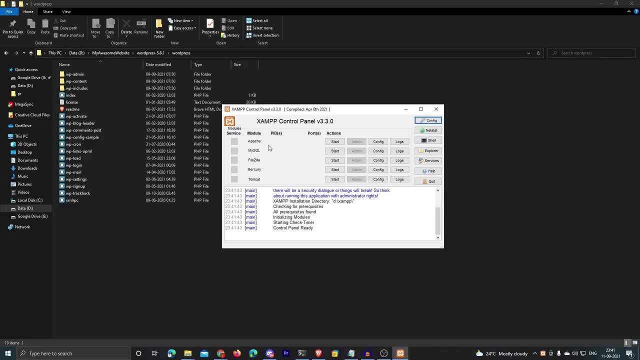 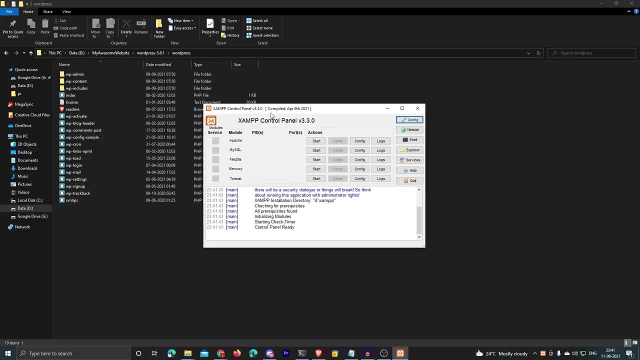 can see, there are different services available. We'll need the first two services, which are Apache and MySQL. Apache, as I said, is a web server. MySQL is a DBMS, So you can just start these two services by clicking on the start button beside them And you can see once they're started. 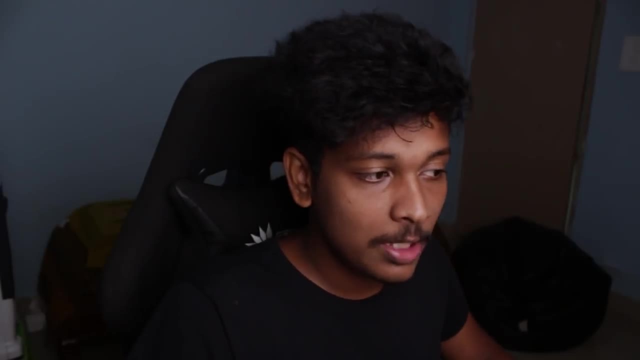 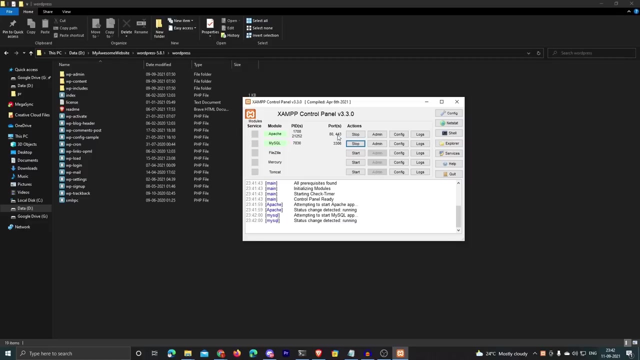 they appear green. And also one thing you need to keep a note of is the Ports on which these services are running. For example, Apache is running on port 80 and 443.. Port 80 is actually the default port of HTTP And, in the same way, MySQL is running on the port 3306,. 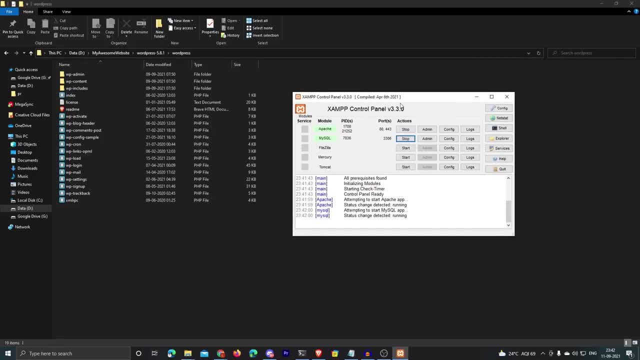 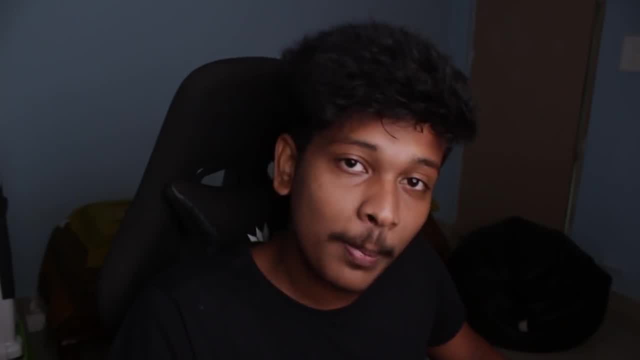 which is also the default port for MySQL. So you can actually change these ports to whatever you like, but I do not recommend changing them because it might bring some complications in other steps that we're going to follow in this tutorial. But if you know what you're doing, then go ahead and 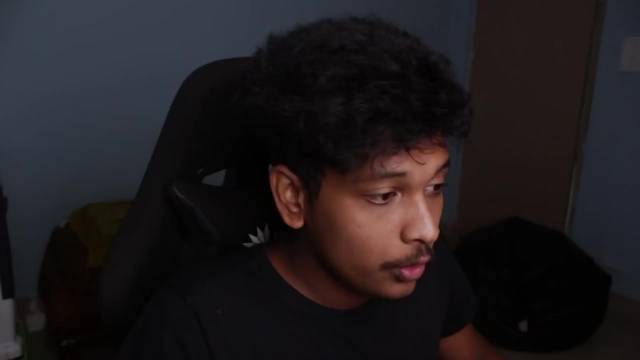 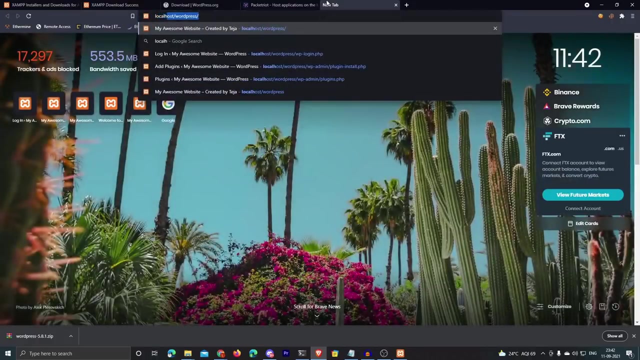 change the ports And I'll see you in the next video. Bye, You can put whatever the port you want, Great. So in order to check if Apache is actually running or not, you can just open your browser and open a new tab and go to localhost And that should bring you a XAMPP default page like this: 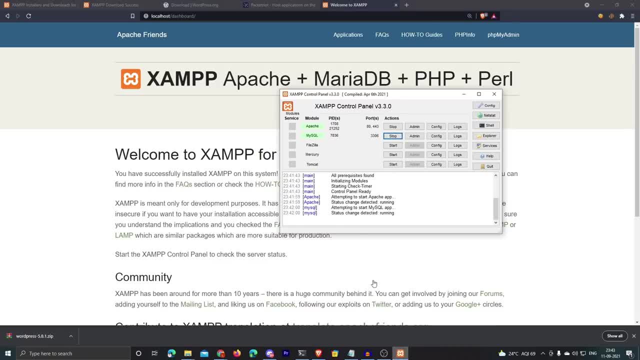 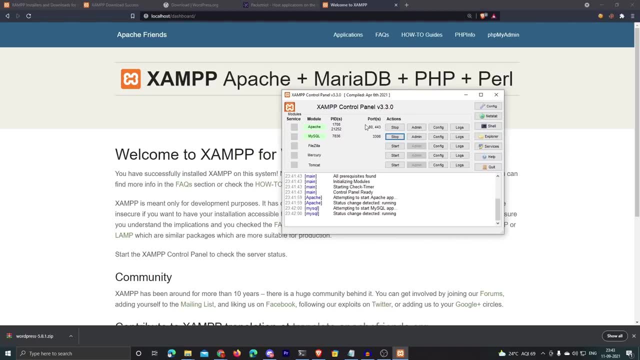 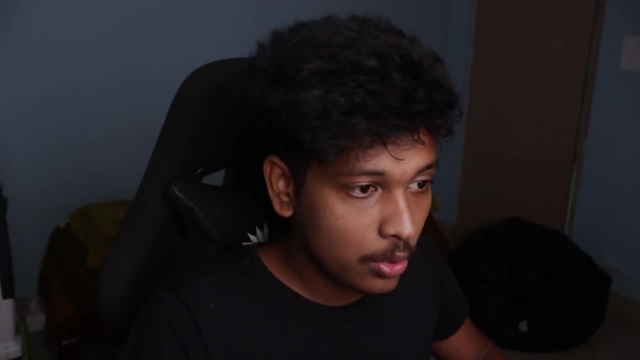 So this: if you see this page, it means that your XAMPP is successfully up and also your Apache is running as expected on port 80.. The next step you need to do is you need to set up the database so that WordPress can use it. In order to do that, just click on phpMyAdmin over here. 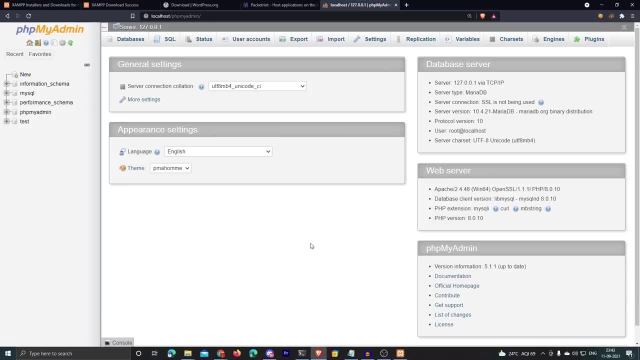 and you will be taken to a web page like this. This is basically an admin console to manage the DBMS, the MySQL DBMS. You can create databases, create tables, create user accounts, et cetera, using phpMyAdmin. It's basically like a web admin console, right? So the first thing you need to do, 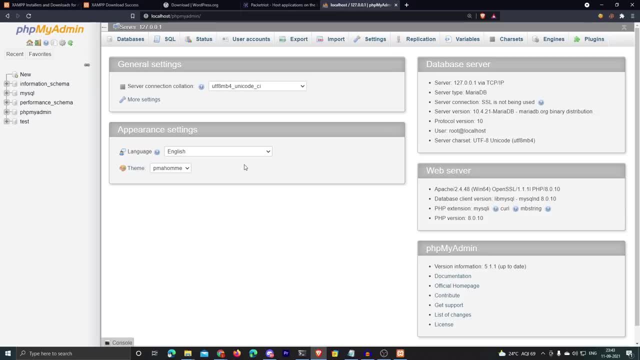 is: you need to create a database for WordPress so that WordPress can use it. So you need to create a database for WordPress so that WordPress can use it. So you need to create a database for WordPress so that WordPress can use it. In order to do that, just click on new here and give the database a. 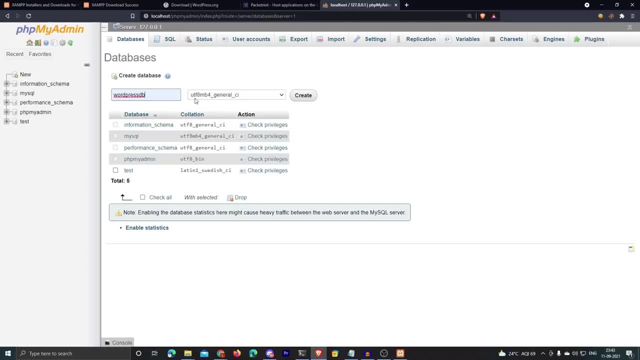 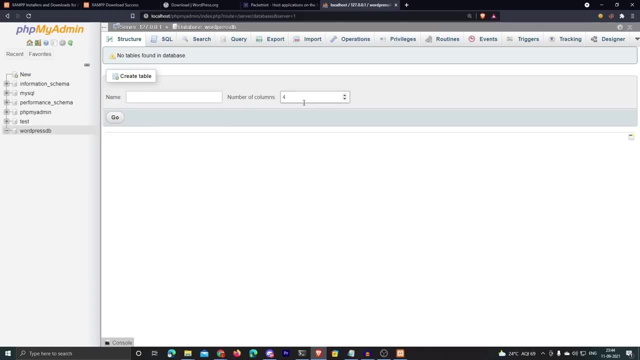 name. In my case, I'm just going to give it a name: WordPress DB. DB stands for database, So click on create and there you go. The database has been created. Now we also need to create user accounts so that WordPress can use these user account to authenticate with the MySQL. 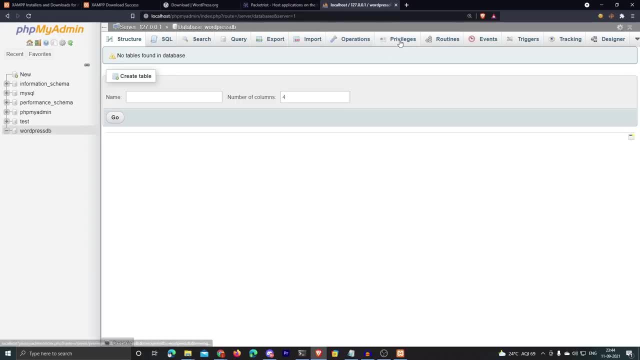 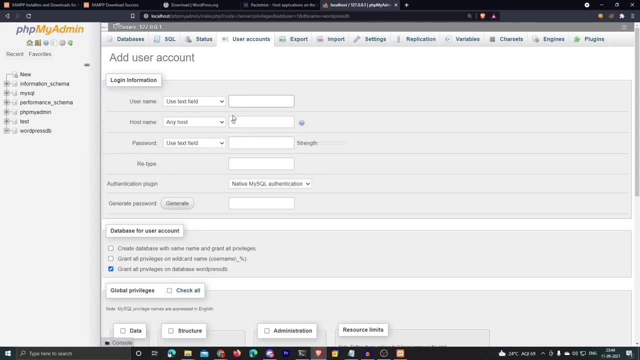 backend database. So, in order to do that, just click on privileges here and on add user account and you can give the username and password. So I'm going to choose the username as WordPress underscore user and I'm going to choose the password as test password. Now you 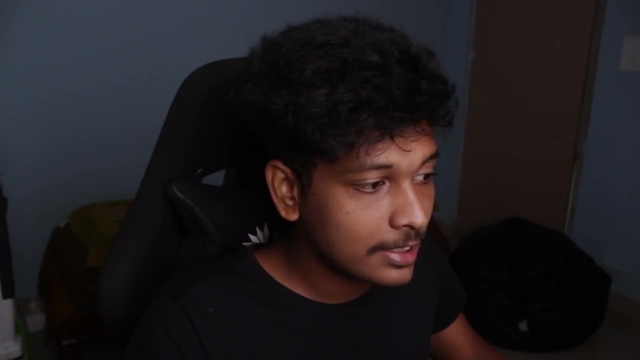 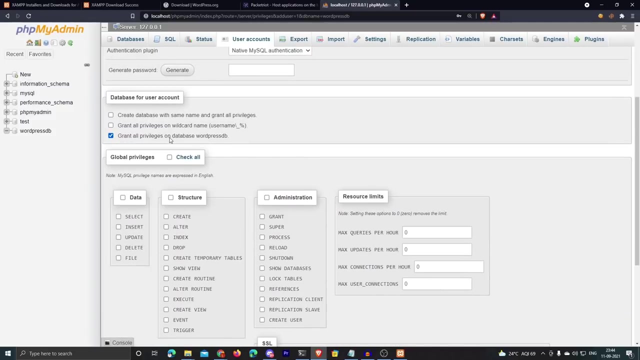 have to choose a strong password in order to stay safe, because if you choose a weak password, like I did here, it is going to be very easy for hackers to crack your password. So make sure you choose a strong password there, And that's it. You just make sure that grant all privileges on database. 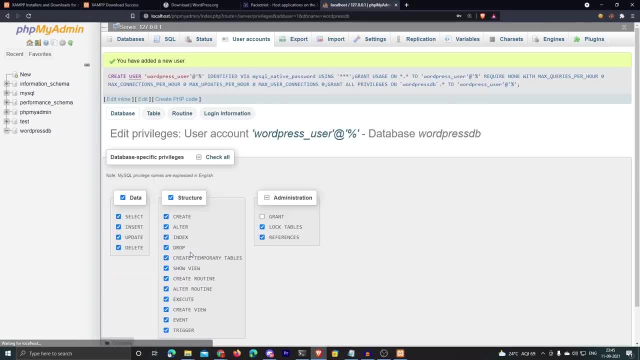 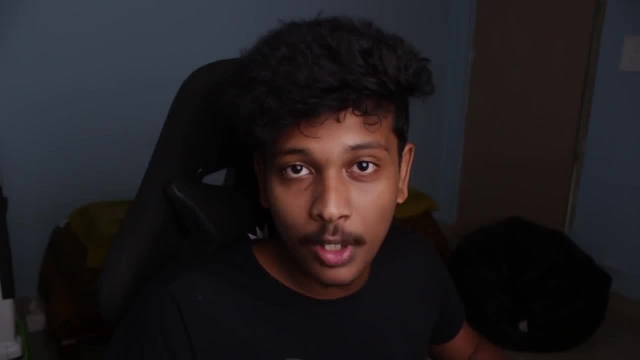 WordPress DB is checked here And finally just click on go. and there you go. It says you have added a new user. Now we are done setting up the database. Now is the time to install WordPress on our Apache server. In order to do that, go back to the WordPress source code files, which. 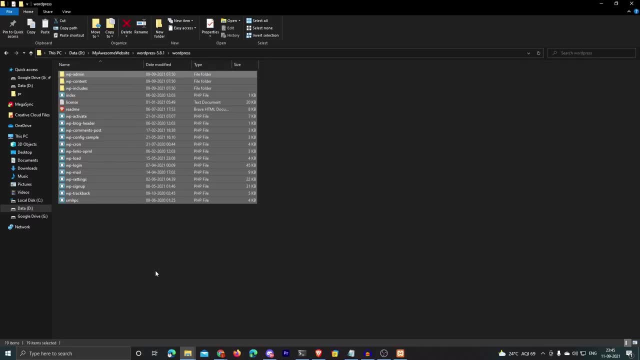 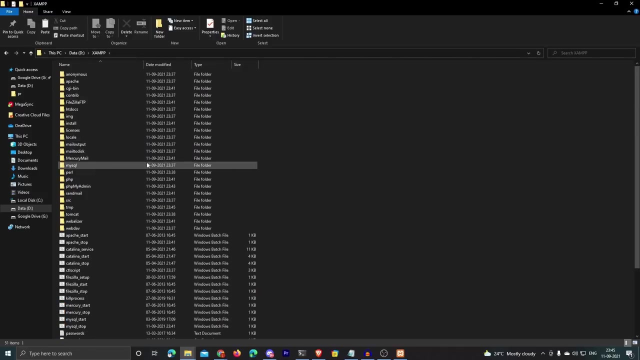 you have extracted earlier. Just select all these files, copy control C to copy and now come to the directory where XAMPP is installed. So in my case it's installed in my D drive in the folder XAMPP. So this is my XAMPP installation directory And inside this directory you will find a folder. 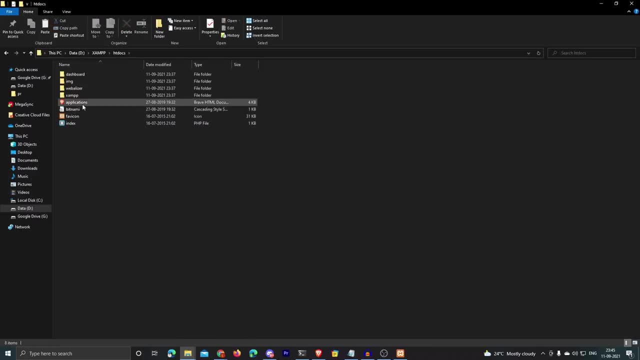 called htdocs. So just go to that folder And over here, just create a new folder. right click, select new and go to folder and name this folder as WordPress, because we are going to install WordPress in this folder. So go to this folder and paste all the WordPress source code files. 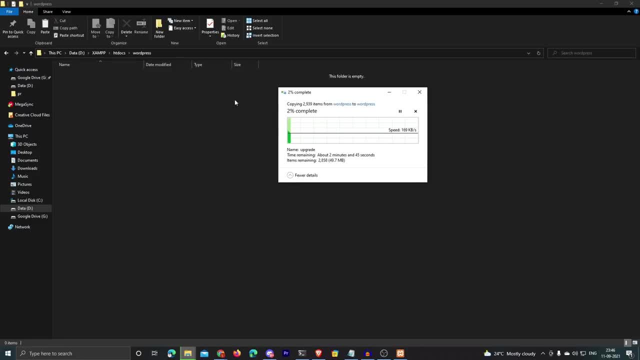 that you have copied. So what we're basically doing is we are installing WordPress in inside this folder and paste all the WordPress source code files that you have copied. So what we're basically doing is we are installing WordPress in inside this WordPress directory. Perfect. 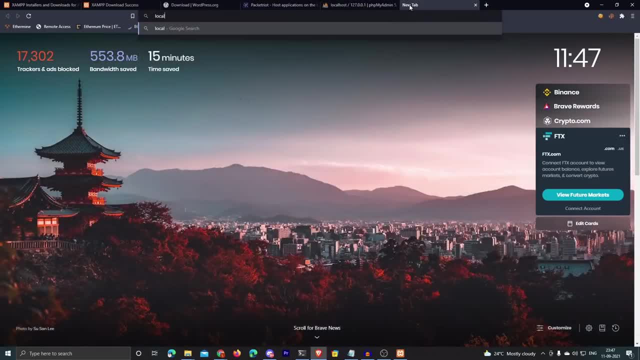 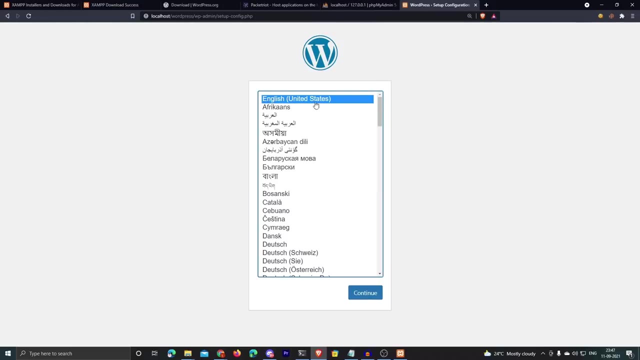 all the files are copied now. So now just open your browser, go to a new tab and type in localhost slash WordPress, And that should bring up the installation page for WordPress. So there you go. Just select your language here. I'm just going to select English. 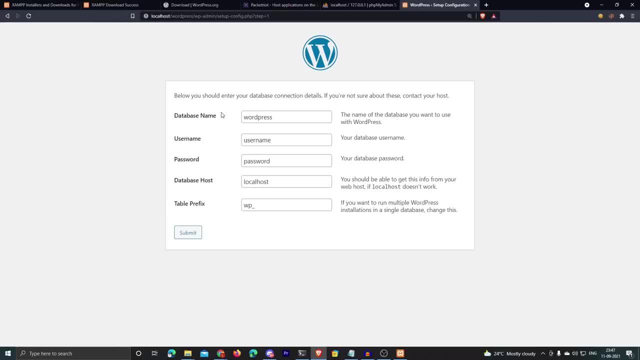 click on Continue And let's go. Now you have to configure the database so that WordPress can use this database. So we have just created a database for WordPress to use. So I'm just going to name the database as WordPress DB, because that's the name. 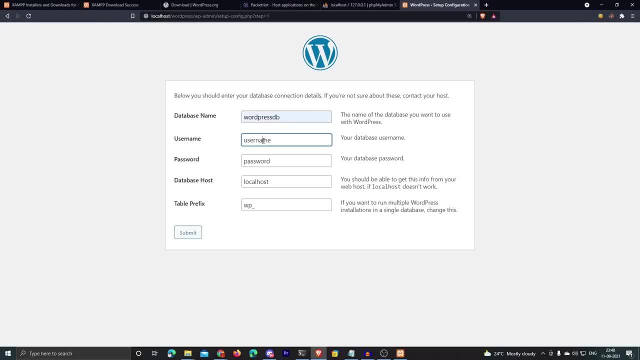 of the database that I've created And the username is going to be WordPress underscore user And the password that I've given is just test password And just leave the database host to localhost and table prefix to WP underscore. click on Submit. click on Run the installation And this should install WordPress. And before doing that, 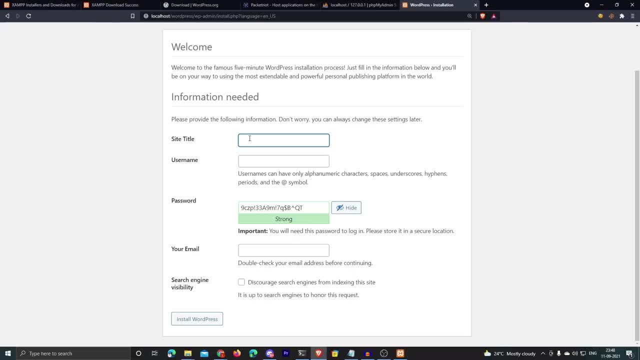 it's going to ask you some details about your site, like the site title, for example. So I'm just going to give this site title as My Awesome Website. I know it's lame, but it works, as I said, And you actually get to choose the username and password that you will use to log into your 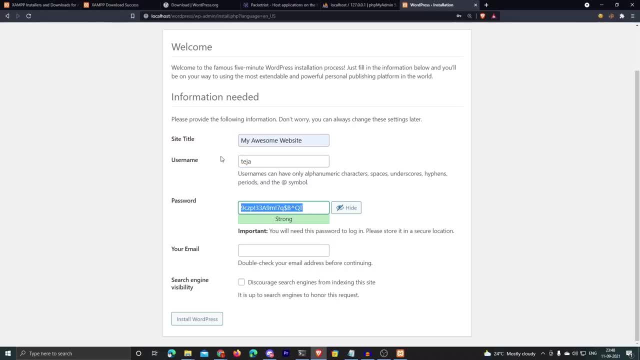 WordPress dashboard here. So I'm just going to set the username to Teja and I'm going to choose a password. By default it's going to generate a strong password. I recommend you use the generated password because it is strong and very hard to crack. But I'm just 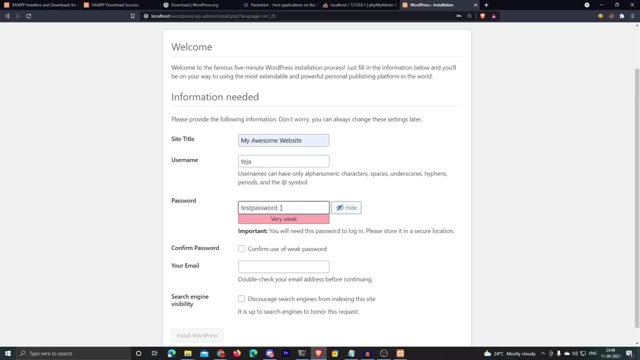 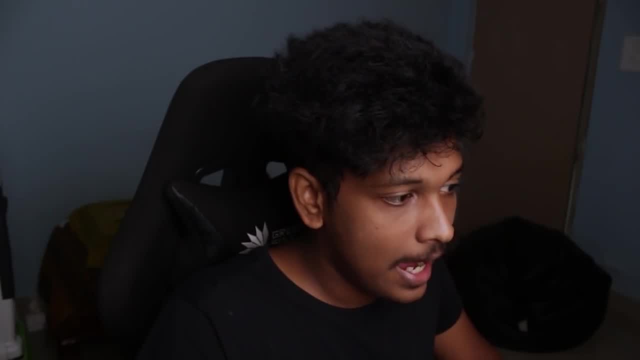 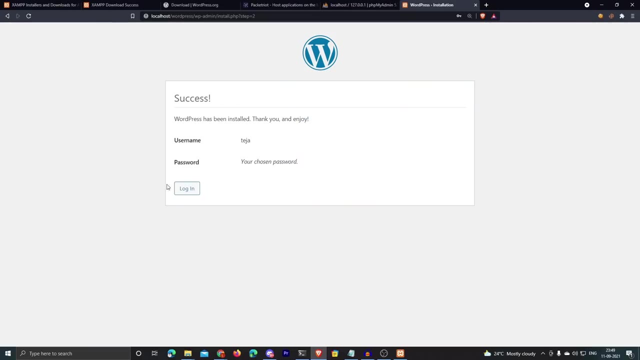 going to use a simple password, like test password, since this is just a demonstration. So put in your password here and click on Install WordPress, And that should take around five to seven seconds to install WordPress. There you go, It says success, WordPress has been installed. So it. 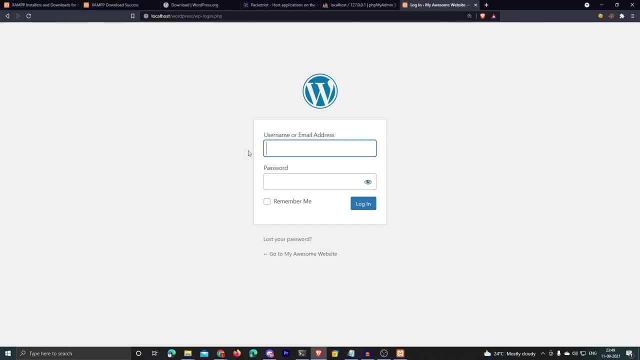 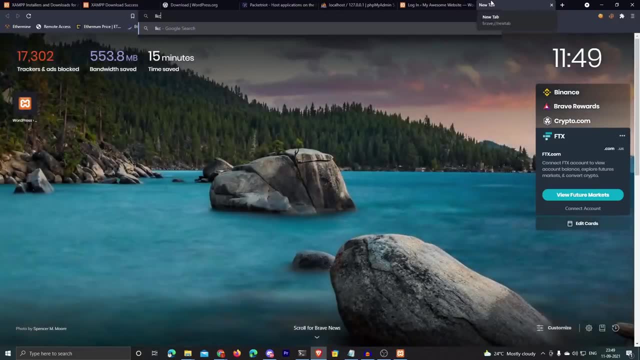 shows you a login button. If you click on the login button, you should be taken to this login page. So this means that you have successfully installed WordPress. So if you open a new tab and go to localhost, slash WordPress again, this time you should see your. 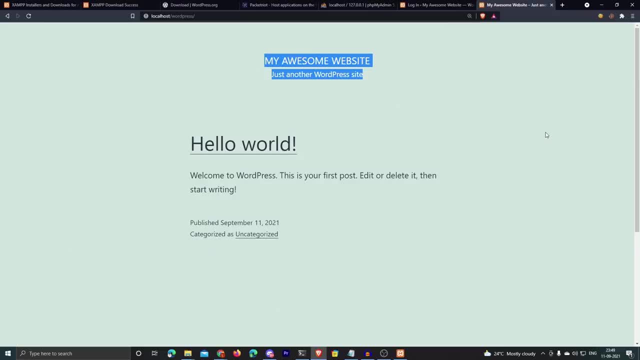 WordPress website. There you go. This is the default WordPress website. Obviously, you can customize it any way you want by logging into your admin console, your WordPress admin dashboard, which I'm going to show. So go back to your login form and log in with your. 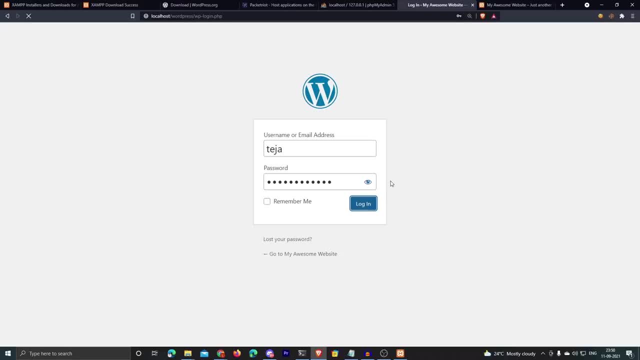 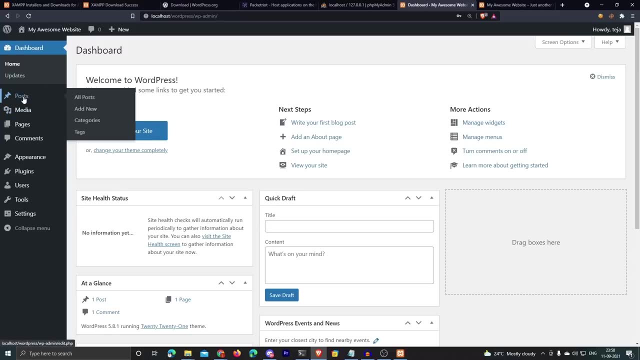 admin credentials, Click login And there you go. This is how the dashboard will look like. So you can do anything. You can customize the site any way you want Using this WordPress dashboard. for example, you can install new plugins, You can add new pages. 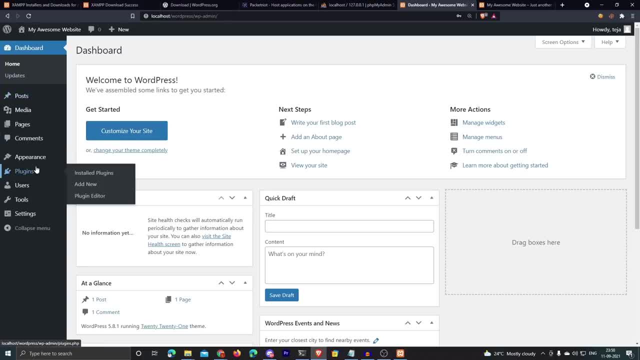 like about page contact page, whatever it is. You can post new blog posts, You can moderate the comments, You can change the theme. Basically, you can do anything. Just going to quickly click on customize your site, And this is going to bring up an editor like this. So over here. 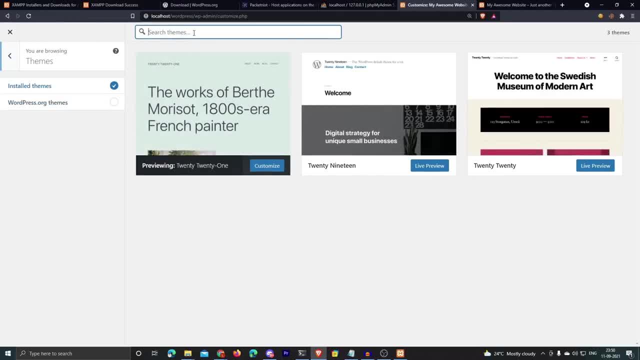 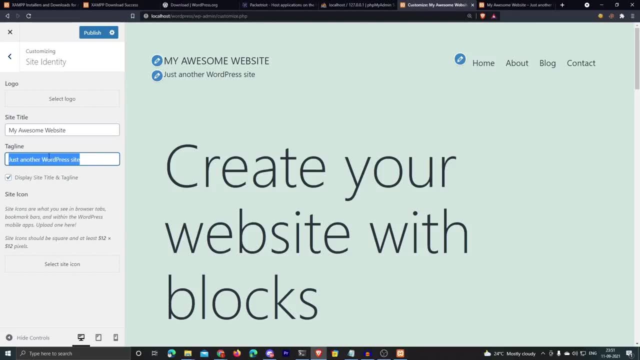 I can change the theme and I can choose whatever theme I like. I can search for themes, whatever. But I'm just going to go to site identity And here I can change my site title And I can also change the tagline. So I'm just going to put the tagline as: 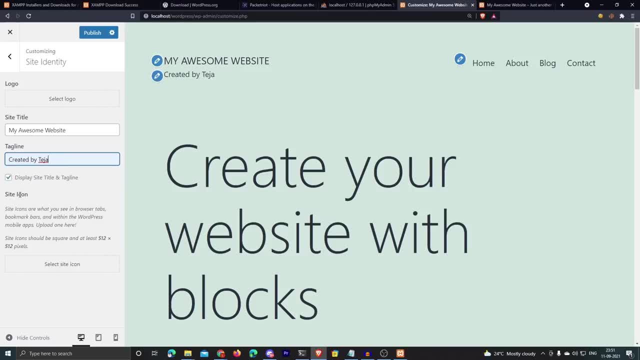 created by Teja, something like that, Because you can also choose the site icon and everything. So once you're done making these changes, just click on publish And the changes are going to be published to the live site. So you get the idea. You can customize the site the way you want. 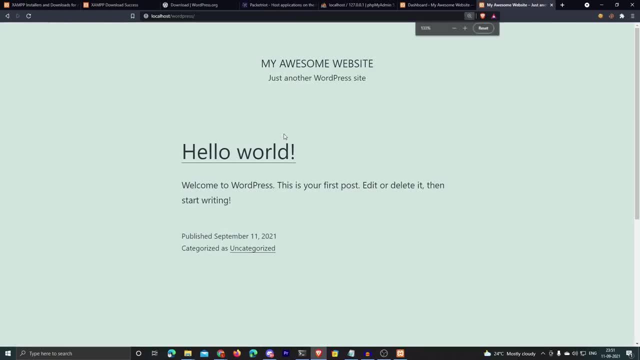 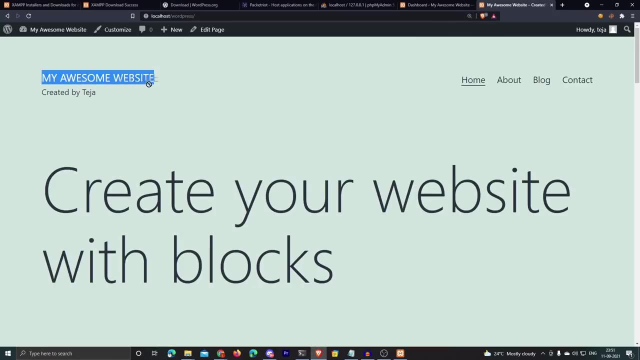 But that is out of scope for this video. So if I just go to localhost WordPress again, there you go: Simple website that I created with WordPress, Perfect. Now you can see that this is actually hosted on my localhost, which means it's only accessible within my network, within my network. 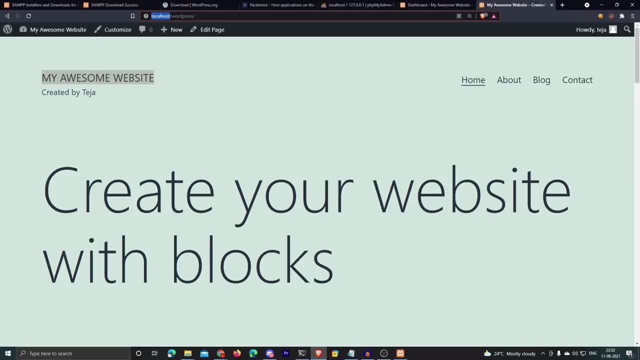 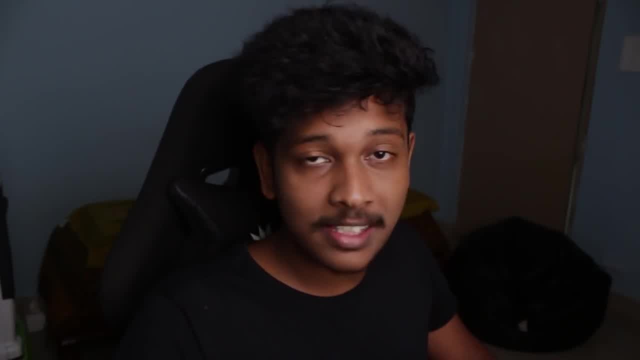 It can't be accessed from outside my network, Or, in other words, it cannot be accessed from the internet. Now, what we're going to do is we're going to make this WordPress website that we just created accessible from the internet. So the first thing you need to do is come back to your 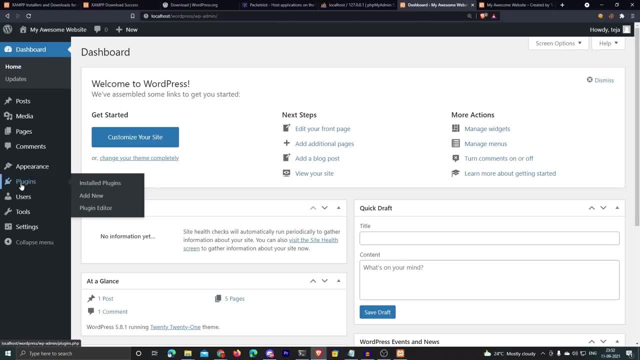 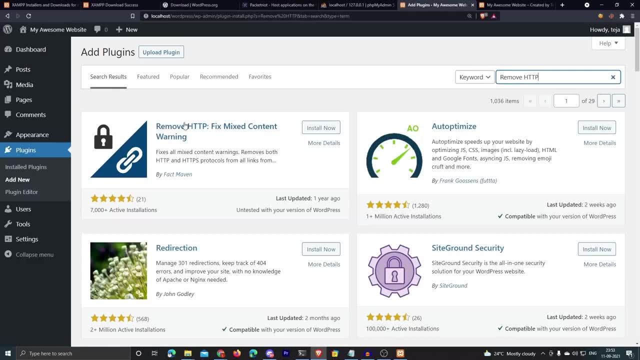 WordPress dashboard and you have to install a plugin. So just go to plugins, click on add new and search for a plugin called remove HTTP. So this is the plugin that you have to install. It goes like: remove HTTP fix mixed content warning. Now it's essential that you install this plugin because if you 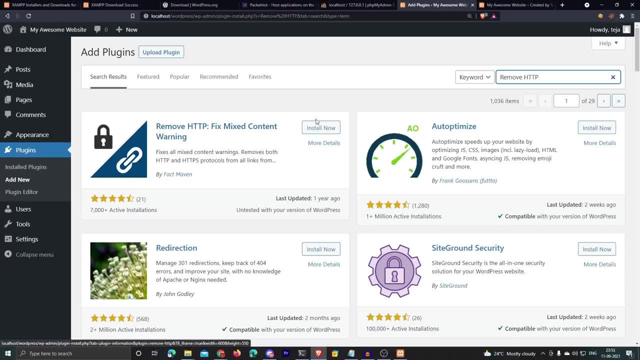 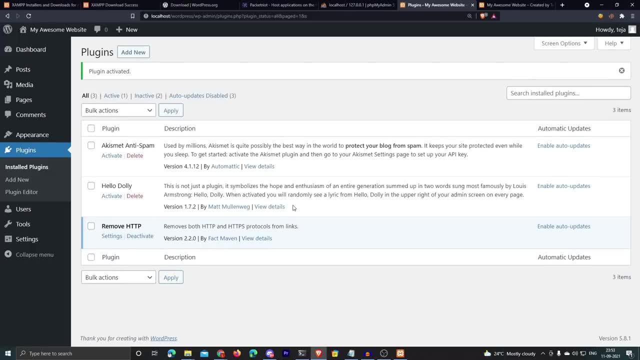 don't install it. you're going to face some issues later. So just click on install now and click on activate, which is going to activate this plugin on your WordPress site. The next thing you have to do is you have to download a tool called as Packet Riot. 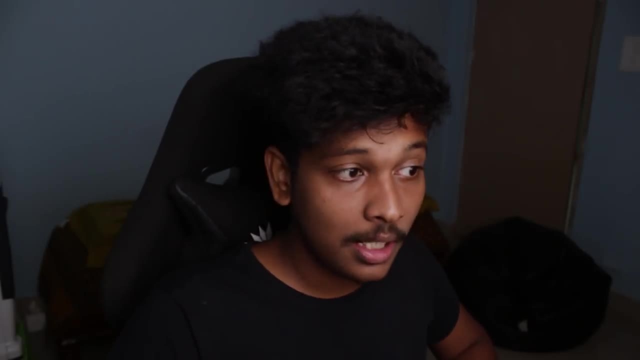 So what it basically does is it creates a secure tunnel from your localhost to the internet. So what we're doing right now is we are hosting our WordPress website on our localhost. So, by using Packet Riot, what we can do is we can create a proxy, or, in other words, a secure tunnel. 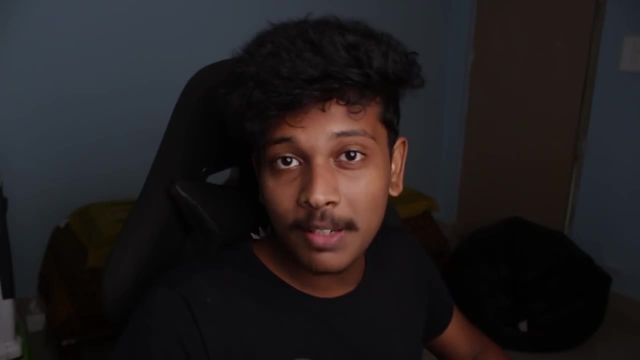 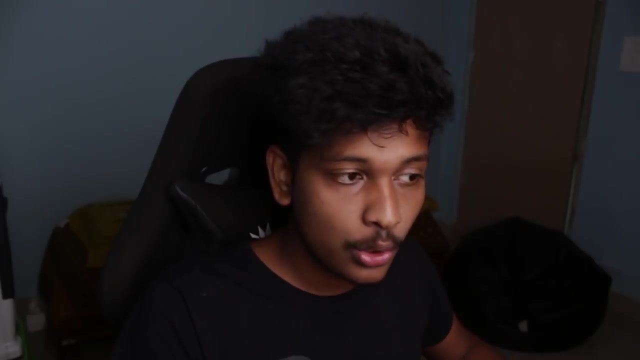 from our localhost to the servers of Packet Riot. So when someone tries to access our website, Packet Riot takes care of proxying all that traffic through the secure tunnel to our localhost. In this way, anyone on the internet will be able to access and interact with the website. 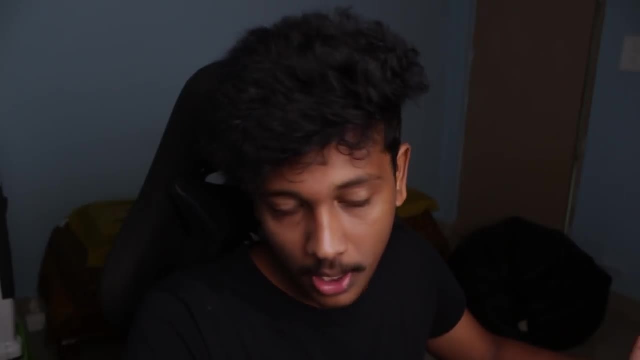 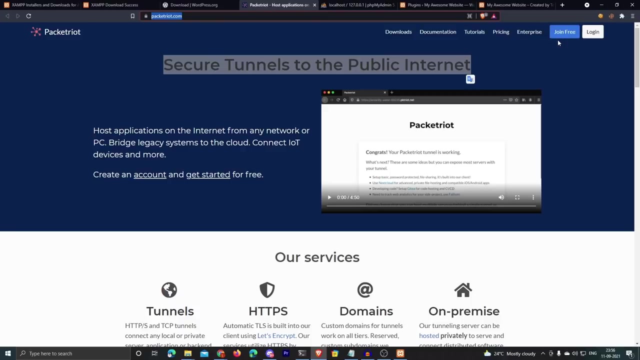 that we are hosting on our localhost, on our local computer. So let's do that. So you can go to PacketRiotcom and sign up for free. It's absolutely free to use. So you can create a new account, And I've actually already have an account. 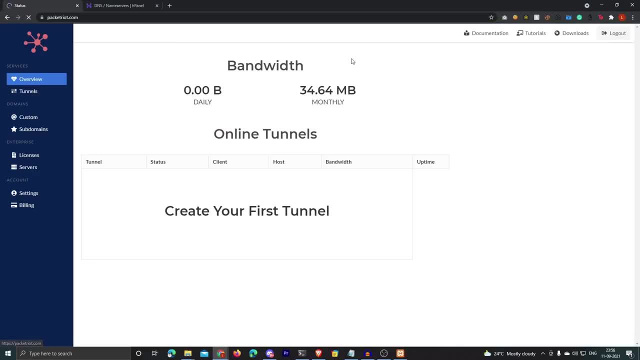 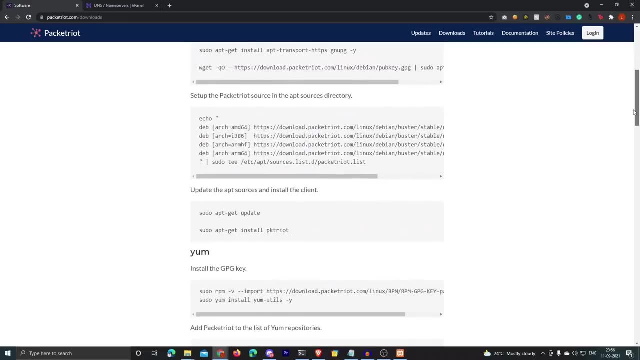 so I'm going to log into my Packet Riot account right now And this is how the dashboard will look like once you logged in. So just click on downloads and it's available for different operating systems. So just scroll down and I'm going to download the Packet Riot for Windows. 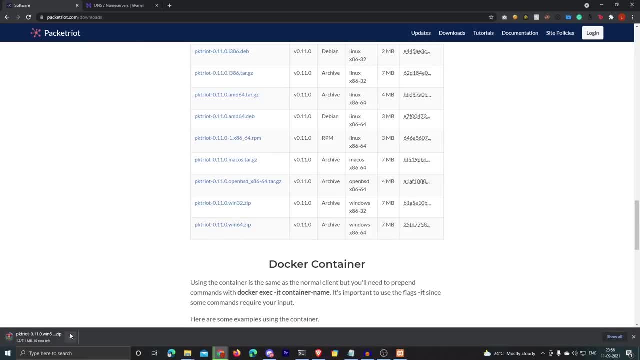 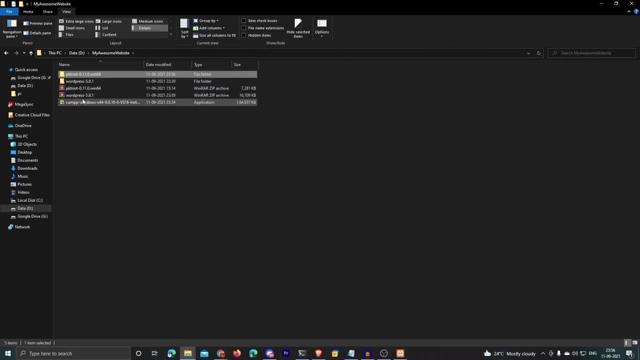 64 bit, So just click on it and that should begin the download. Awesome. Now I'm just going to extract this downloaded zip file using 7zip And, if I go inside this directory, this is the PacketRiotexe file, which is the actual tool that we'll be using Now. I recommend you to add this. 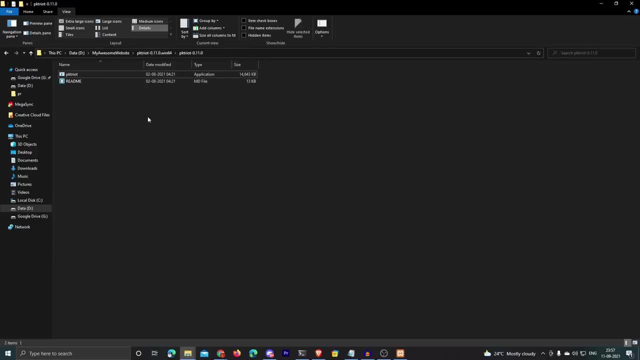 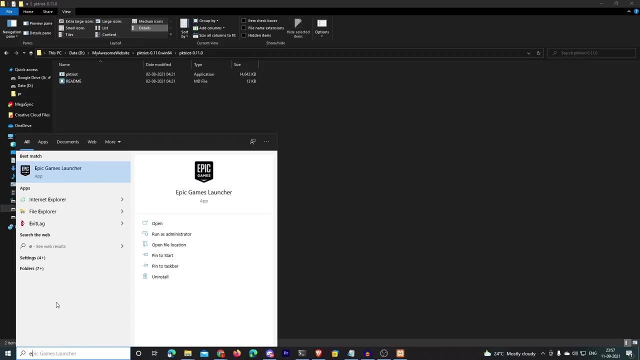 to your path variable so that you can access this tool from any directory. So in order to do that, select this path right click, copy, go to your start menu and search for environment variables, And you will see an option that says edit the system environment variables. 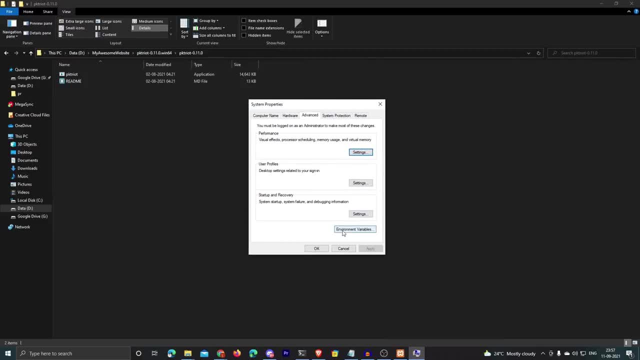 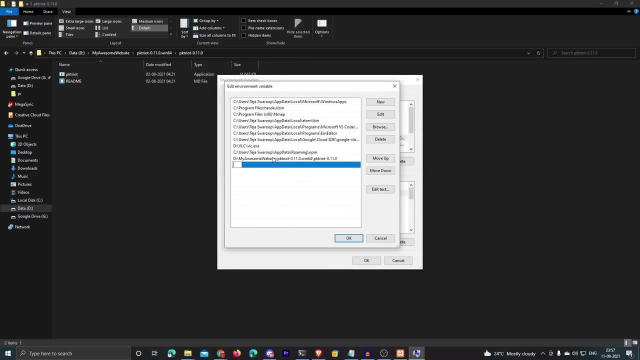 So we click on that. a pop up like this comes up and then click on environment variables. Under user variables, select path, double click on it and here click on new and paste the path to the PacketRiotexe file here. Click OK, OK and OK again. 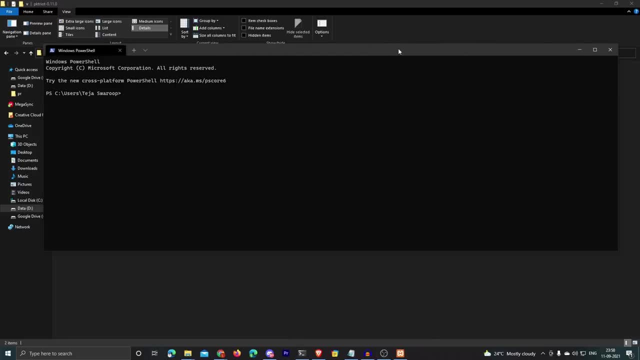 So now, let's go ahead and create a new account. So let's go ahead and create a new account. So now, let's go ahead and create a new account. So now, let's go ahead and create a new account. So if you open your Windows Terminal or the command prompt and if you type in packet riotexe. 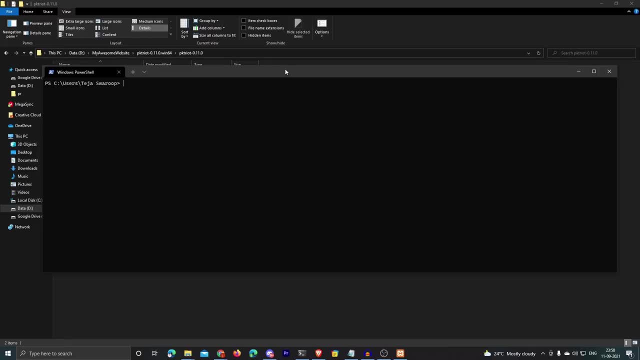 you should see usage instructions like this. So the first thing you need to do is you need to configure PacketRiot. In order to do that, just type in packet, riotexe, space configure And select the path to the configuration file, And then you need to authenticate with your login credentials. So I'll just log in. 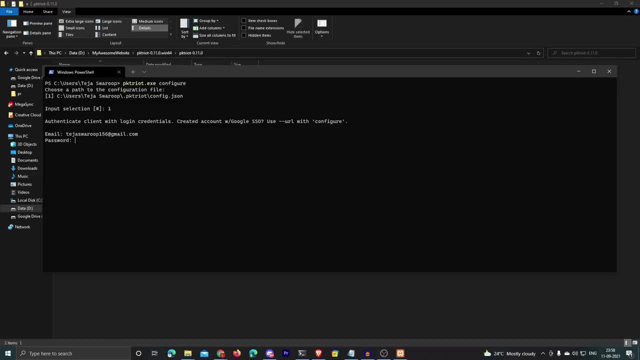 with my credentials here. So there you go. it says authenticated. And now is the time for you to choose a region which is geographically closer to you. So I'm going to choose Asia, Southeast here. And that's it, Great. So the configuration is done. It will also show you the host name. 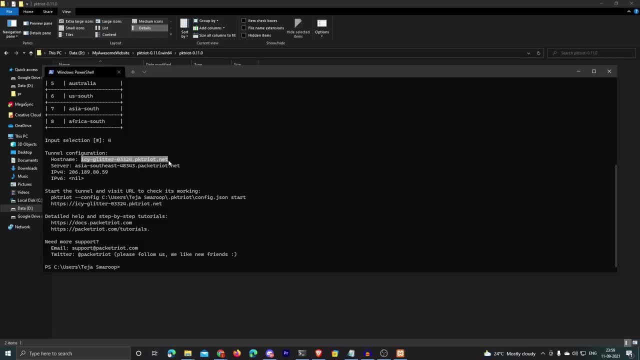 which is going to be unique for you. So this is not going to change. this is basically assigned to you. it's a unique host name assigned to you And we'll actually need this host name to do stuff. So next thing you can do is you can change the name. 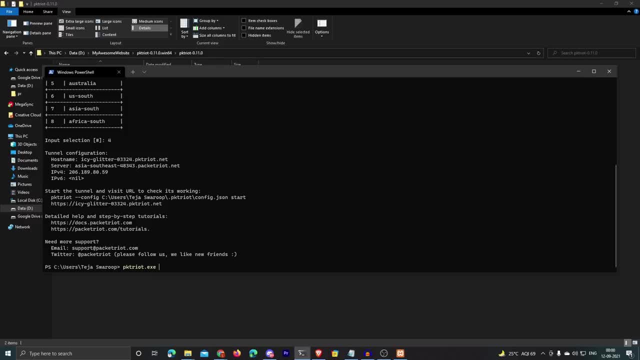 of your tunnel In order to do that type in packet, riotexe, space, Edit, space, dash, dash name and then followed by the name you want to give to your tunnel. So I'm just gonna say the name as WordPress underscore tunnel And if I hit Enter. 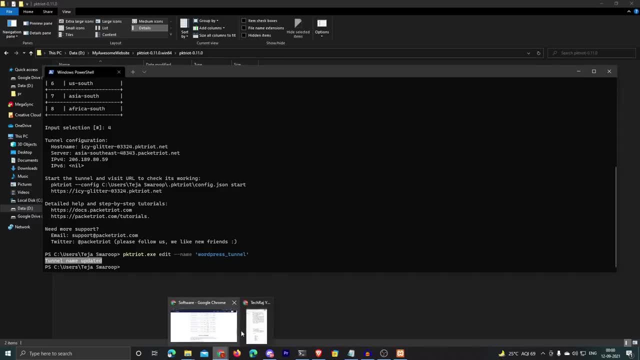 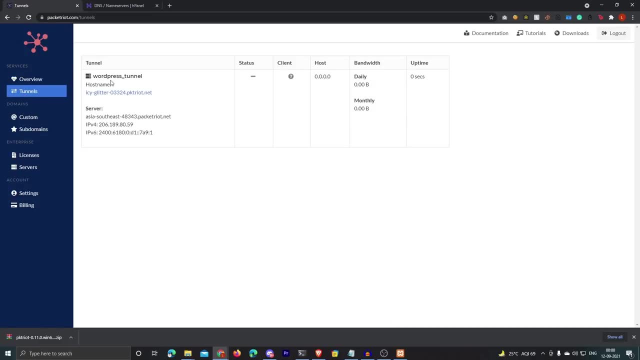 there you go. it says tunnel name updated. in order to cross check this, if you go to your packet triad dashboard, go to packet dashboard, go to tunnels, you can see there is a tunnel named wordpress underscore tunnel and you'll also be able to see the host name. so now comes the moment. 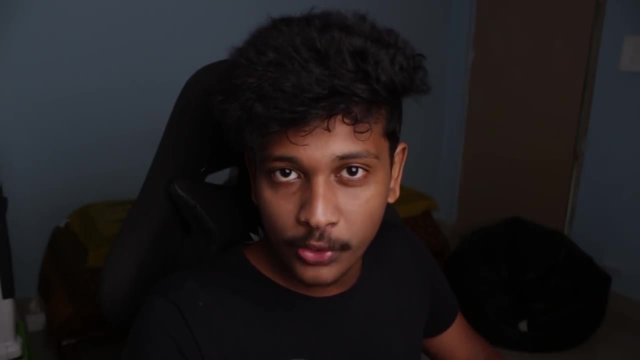 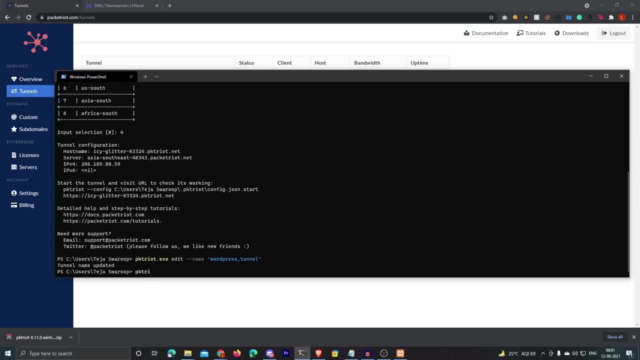 of truth, we need to now expose our local host to the internet so that anyone can access our wordpress website. so in order to do that, you just have to add a http service to the packet triad tunnel that we have just created. so just type in the command: packet- ryotexe- space tunnel. 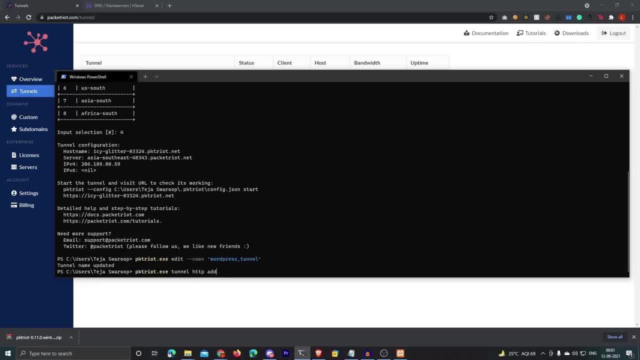 http, add dash dash domain, and then mention the host name that is assigned to you, which in my case is this. so i'll just copy this, i'll paste it here: space dash dash destination local host, because that's where our wordpress site is running. space dash http, and then port 80, because 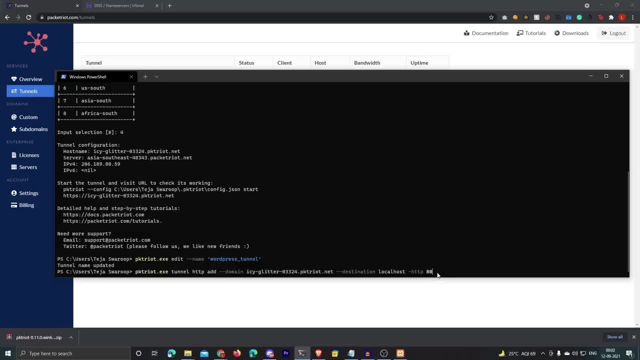 port 80 is the code that we're using for our local host. so if you want to copy this code, 80 is where our apache server is running, and followed by dash, dash, let's encrypt. so we are using let's encrypt to enable ssl, so that our url will be https or not just http, so it will be more. 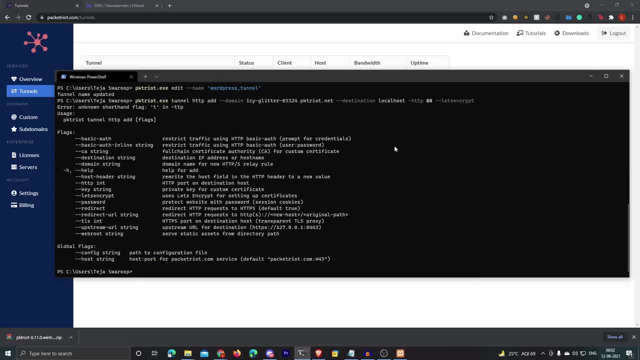 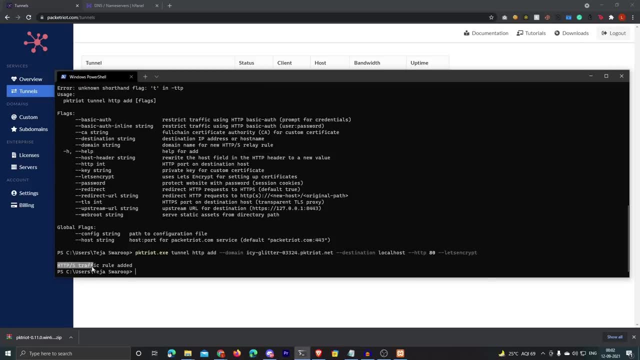 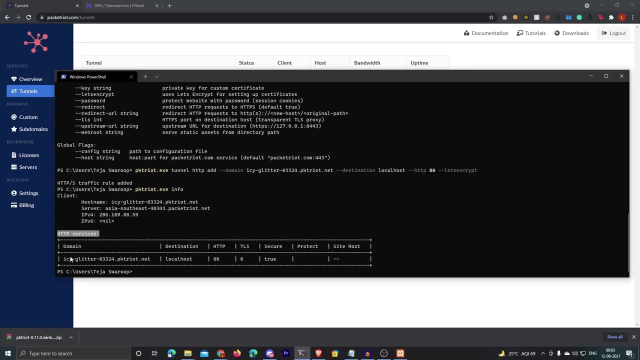 secure. so if i hit enter, um, it seems like we have missed something. oh, it's actually going to be dash, dash http. if i hit enter, now there you go. it says http traffic rule added- perfect. so if i say packetriotexe space info, you can see that the http service is added with the domain, which is: 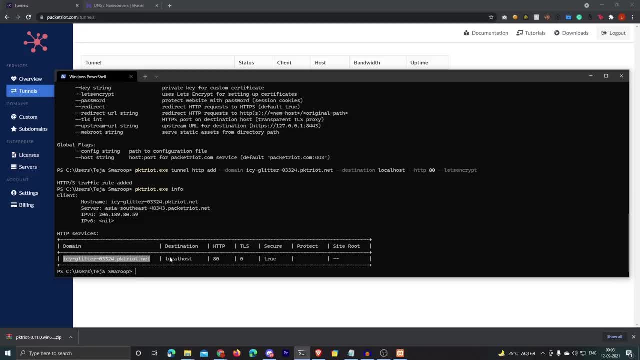 basically just the unique host name that is assigned to you by packetriot and you can see the destination is local host, the port is 80. so now, in order to start packetriot, just type in packetriotexe, space, start, and that should take a little bit of time to start the packetriot. 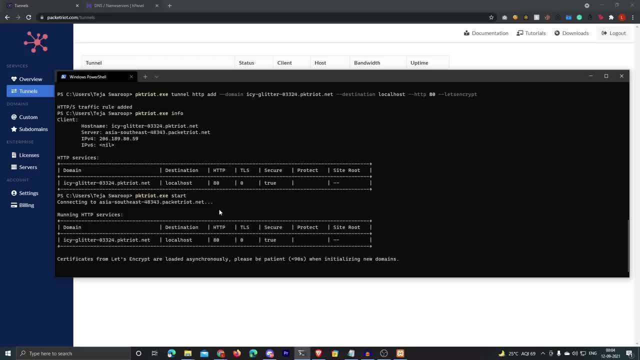 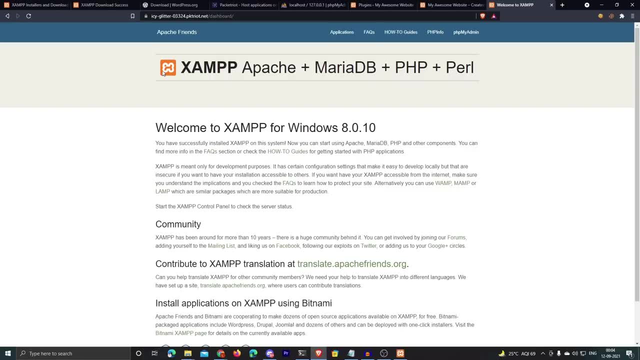 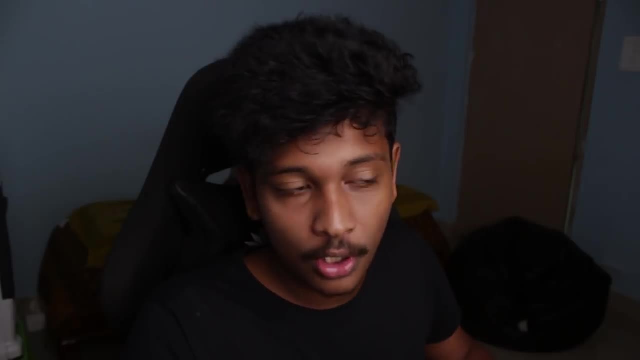 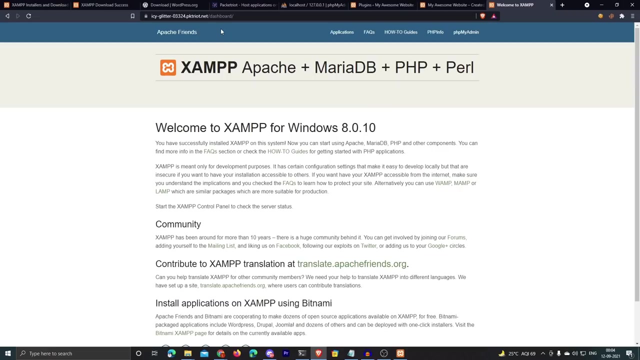 this means that my local host is successfully exposed to the internet. now i can access my local host from anywhere on the internet. perfect, but what about our wordpress site? so in order to access the wordpress site, you have to go to slash wordpress, because we installed it in a subdirectory. 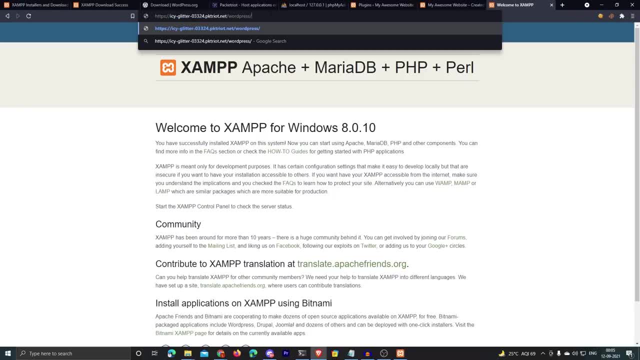 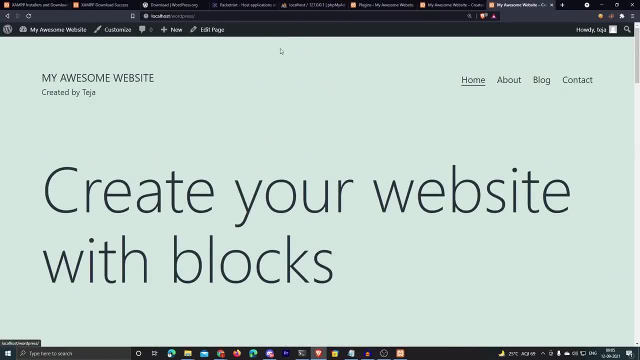 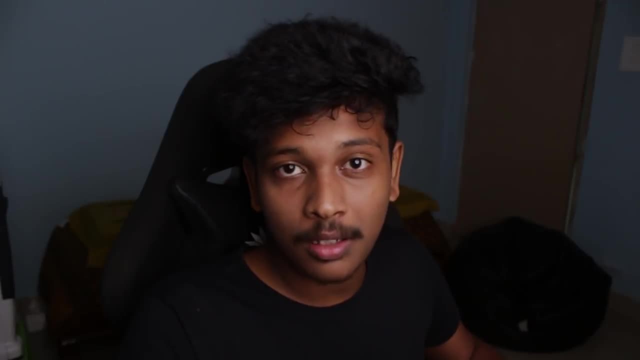 called wordpress. so just go to your domain name, followed by slash wordpress, and that should bring you your wordpress website. but something is wrong here. if you could notice, you can see that the url is just localhost- slash wordpress. well, this means that we are not actually accessing our wordpress website from the internet. 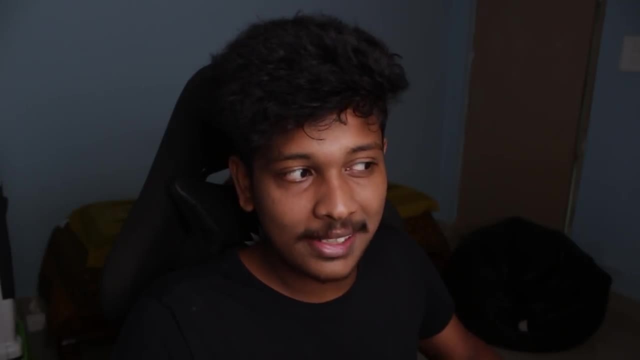 we are just accessing on our localhost, which is not exactly what we want, right, because we want to access our website from the internet, not on local. in order to fix this, you need to make some changes with the wpconfigphp file. so just open your xampp directory and come to history docs. 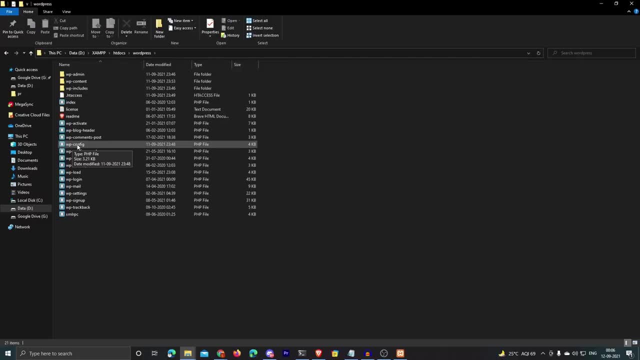 go to wordpress and then go to your zamp directory and you will see that zamp directory is not actually, and you will find a file named wp-configphp. So just open it with any text editor you like. I'm opening it with brackets. 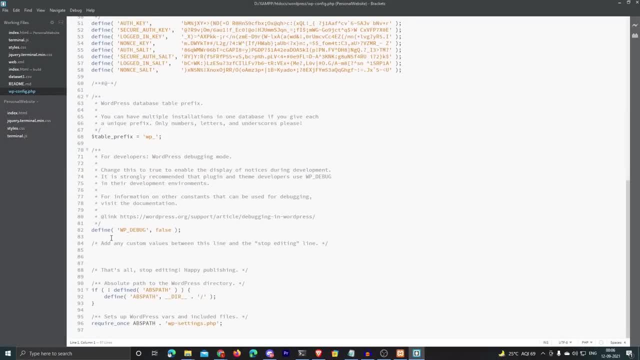 And over here you will find a comment that says add any custom values between this line and the stop editing line. So in between these two comments we need to actually declare two define statements. The first define statement is going to be define wp underscore home. 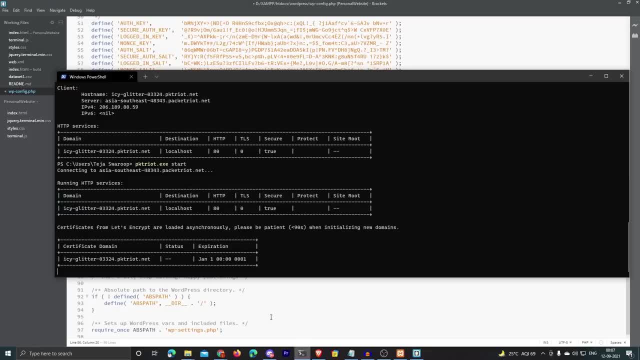 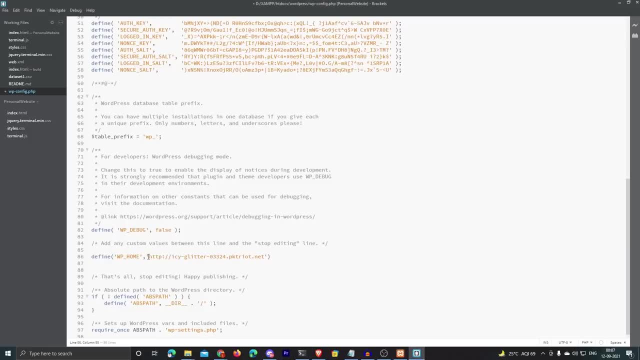 and we are going to define it with our host name, which is icglitter something. So just copy your host name here and just say http//, followed by your host name, followed by a slash- WordPress. So, basically, what we're doing is we're assigning. 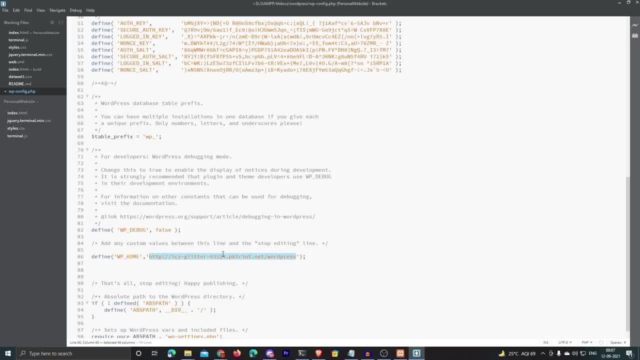 the WordPress home to this URL, so that the WordPress knows that its URL is this. And the same way we're gonna do another define statement. this time we're gonna say wp underscore site URL and we are going to give the same URL for this as well. 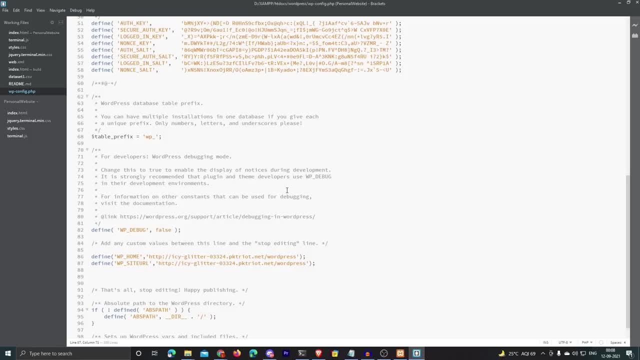 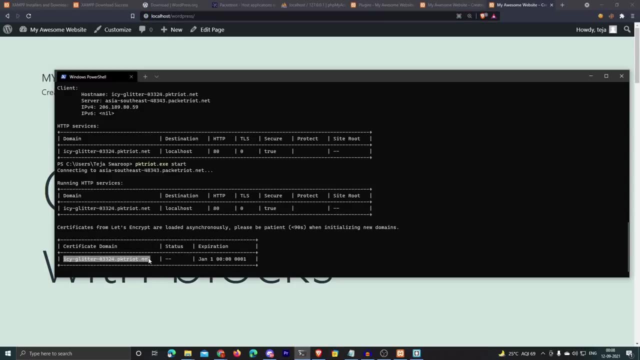 And that's it. and that's it. Once you're done, just save it. control S to save. and now, if you go back and go back to your host name, to your domain, I'll just copy this and paste it in my browser. 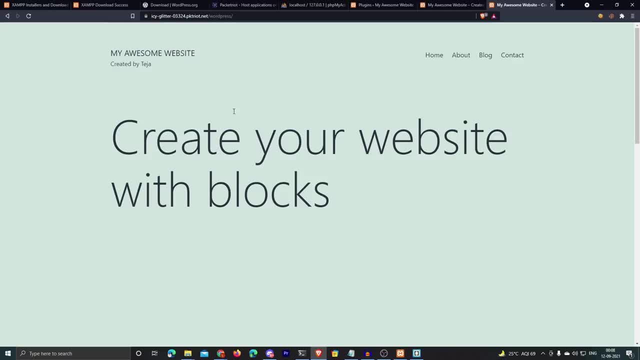 and I'll say: slash WordPress at the end. And this time, as you could see, we are able to access our WordPress website And you can have a look at the URL as well. We are actually accessing it from the internet, from the domain name that is given to us by packet tryout. 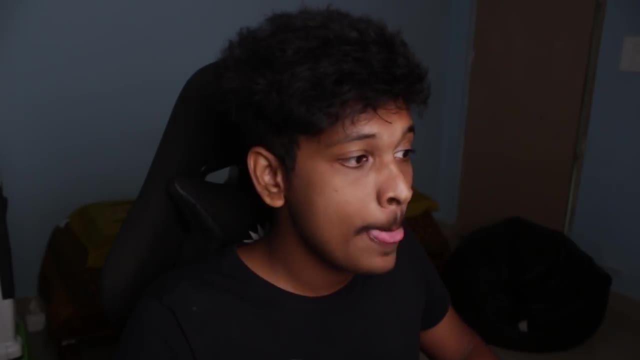 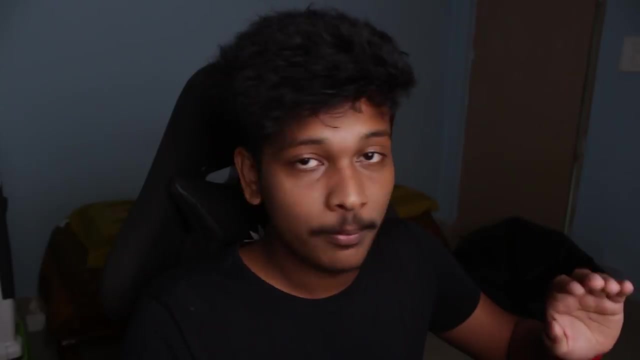 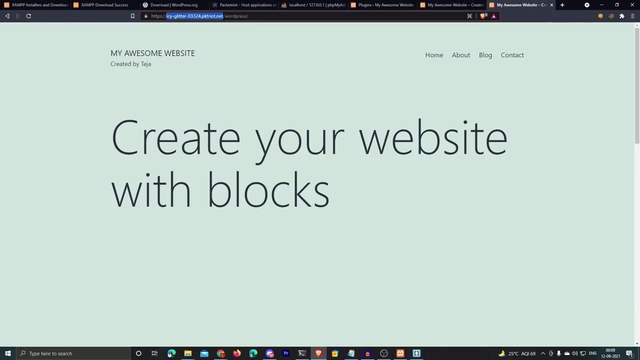 How cool is that We are not hosting our website on any hosting provider. We are hosting it literally right from our computer and people are able to access our website from the internet. That's cool. right Now, you might ask what if you want to change this domain name? 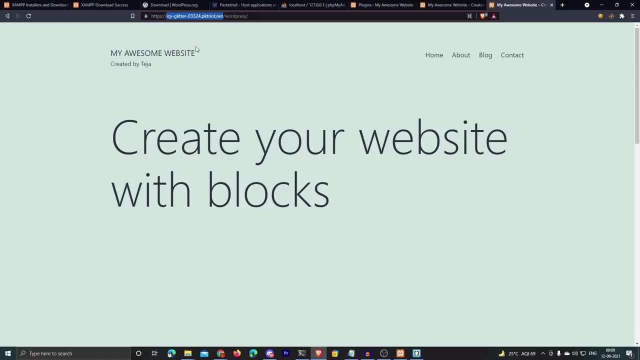 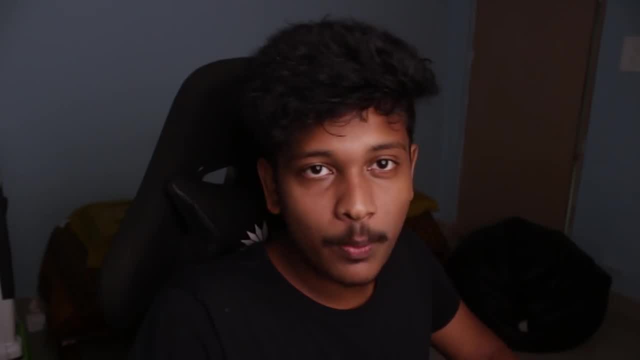 What if you want to use your own custom domain name? Well, that's absolutely possible, But before doing that, you obviously need to have your own domain name. So I went ahead and I purchased a domain for myself. The domain is mylocalsiteonline. 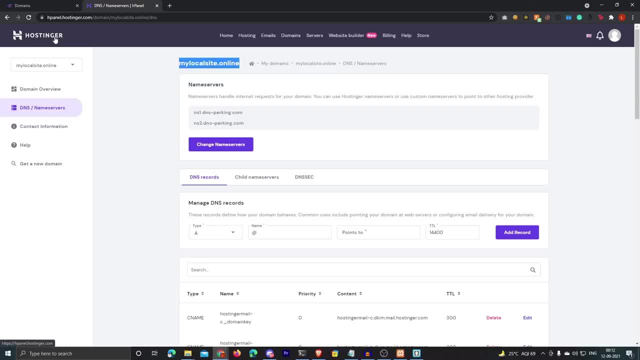 I purchased it from Hostinger and it costed me like 75 rupees for one whole year, which is very cheap. It's like one dollar for one whole year, which is awesome. But you can also get a free domain at freenom or any other services you would be able to. 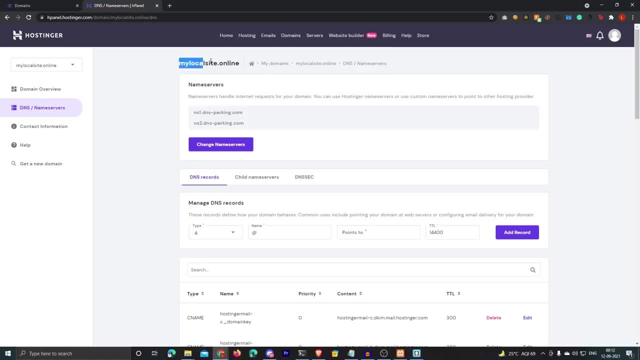 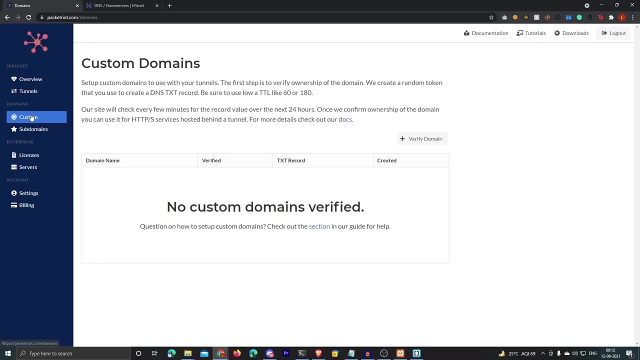 be aware of. so you need to change the dns settings of your domain in order to link it with packet riot. in order to do that, just go to your packet riot dashboard and click on custom, and over here, click on verify domain and just enter the domain which you own, which, in my case, is my local site. 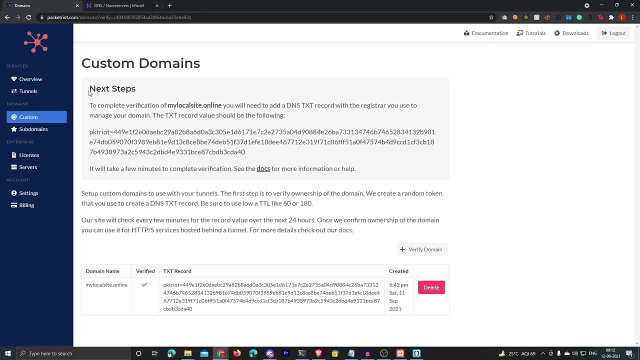 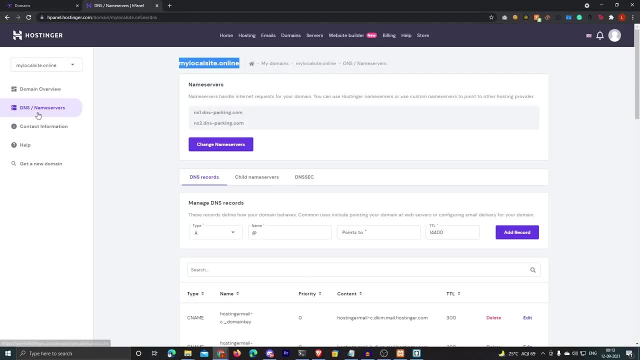 dot online and click submit, and now it will show you the next steps that you need to follow, and basically, what you have to do is you have to copy this text right here and go back to your dns settings on your domain provider- domain name provider in this case. in my case, it's hostinger. 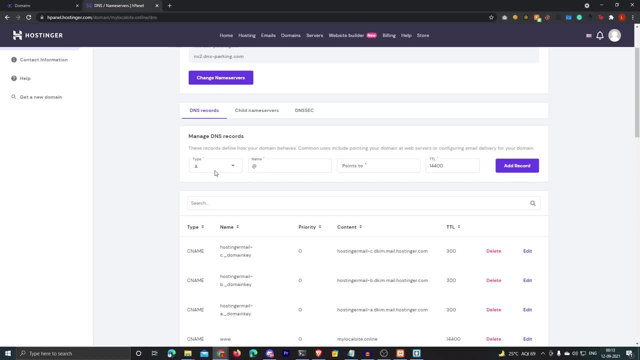 come to your dns settings, and here you have to create a new dns record with the type txt, and for the name just let it be as at the rate, and for the txt value just paste the string that you copied from the packet riot dashboard, and for the ttl put it as 60 and click on add record. so what this is. 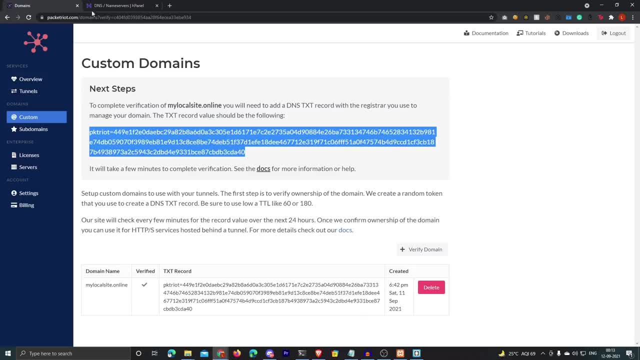 going to do is. it's basically going to link your custom domain with packet riot so that you can use it with your wordpress website or whatever the site you are trying to host from your local host or your local computer, in other words. so you have to wait for. 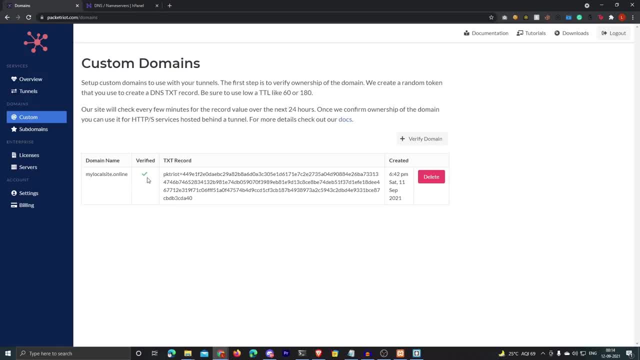 some time until these dns changes propagate. and there you go. it shows a green tick symbol, which means the domain is successfully linked with packet riot. now we can use it for our website. so before doing that, i'm going to first create a sub domain for my domain. so i'm going to go back. 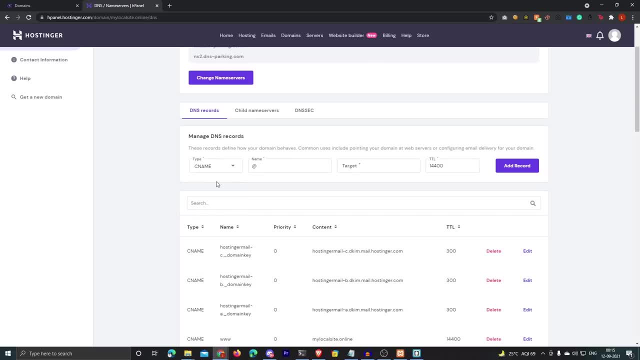 to my dns settings and this time i'm going to add a cname record and in the name i'm going to put it as wordpress, because i want my subdomain to be wordpressmylocalsiteonline, so i'll put wordpress here. you could put whatever you want there and for 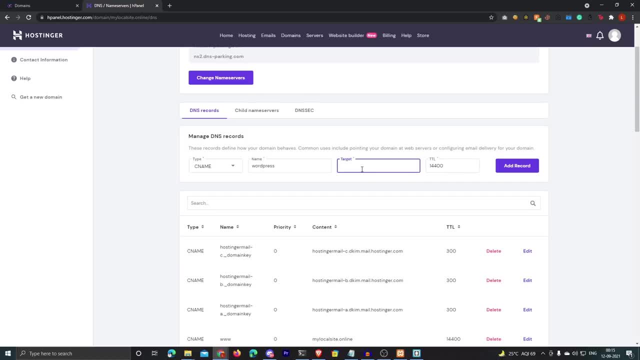 the target. you need to insert your host name, the host name that is given to you by packet riot. in my case, it is going to be this one, so i'm going to copy this host name, i'm going to put it in target and i'm going to put this as 1800, the ttl, and click on add record. 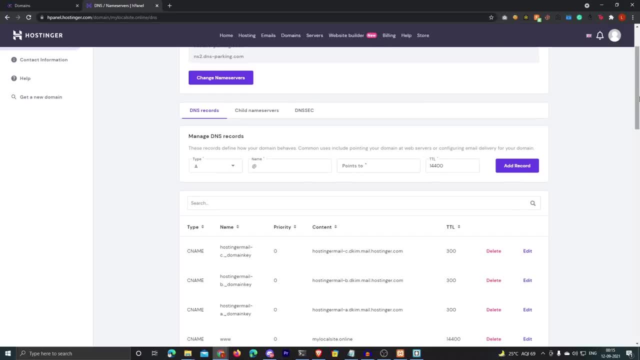 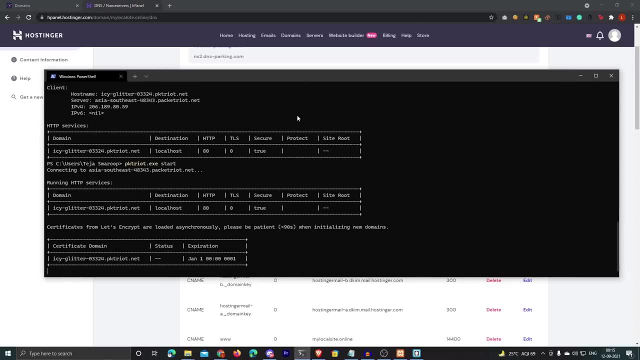 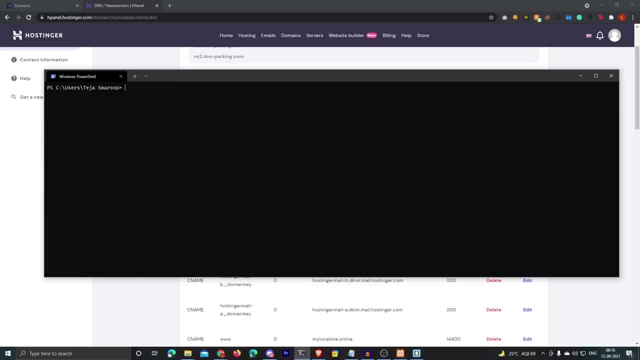 um, that's it. so now we can assign this subdomain, wordpressmylocalsiteonline, to my wordpress website and in order to do that, i'll go back to my windows terminal. i'll stop my packet riot and i'm going to add another packet riot, http service. so i'm going to say packet. 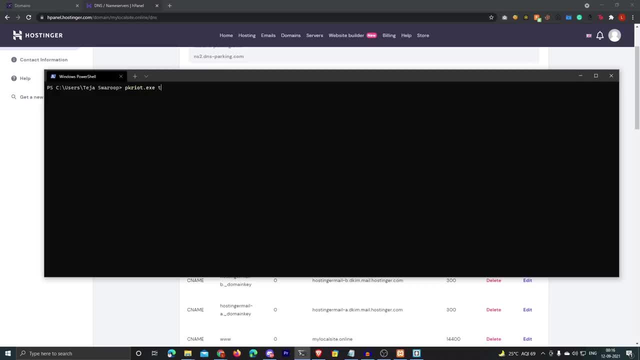 riotexe space um tunnel http. add dash dash- domain, and in this case my domain is going to be mylocalsiteonline, followed by destination, which is localhost, and then dash dash- http and the port 80, which is where apache is running on, and then dash dash- let's encrypt so that we get a https. 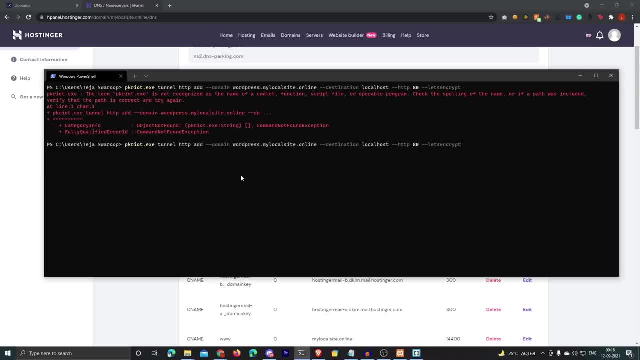 so if i hit enter: um, okay, it seems like i misspelled packet riot there. i'm gonna fix that error. there you go. it says http traffic rule added. so if i say packet riotexe info, you can see that we have successfully added a new http service with the domain wordpressmylocalsiteonline. so this is the custom. 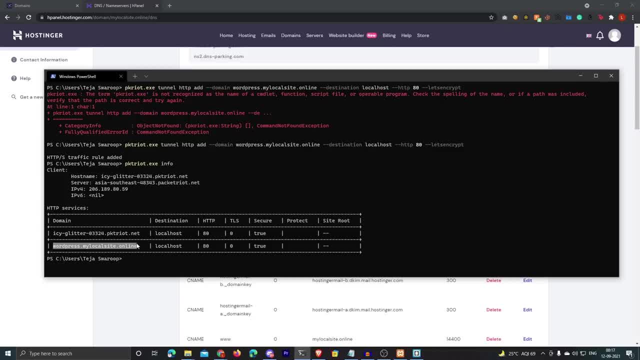 domain that we are using. this is the domain that we own and we are using for our wordpress website. so, in order to start packet riot- you already know how to start it- just say packet riotexe, space start and that's going to start packet riot. so packet riot has started and we are going to start packet. 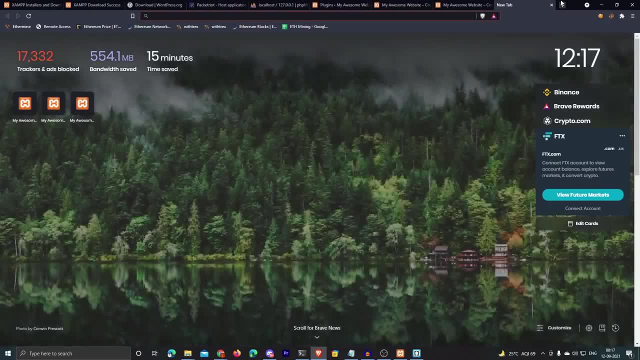 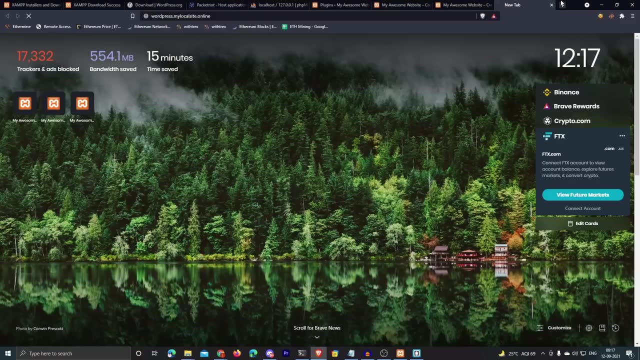 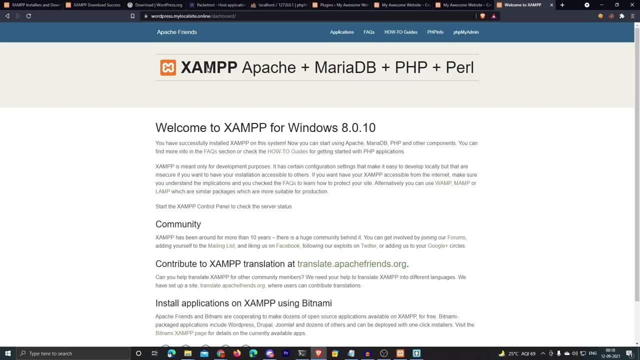 riot. i'm going to go ahead and check if this is actually working or not. so i'll just go to wordpressmylocalsiteonline and i'm going to hit enter. there you go. um, it shows you the xampp default page. but we know what this means, right? this means that our localhost is exposed and we are able to. 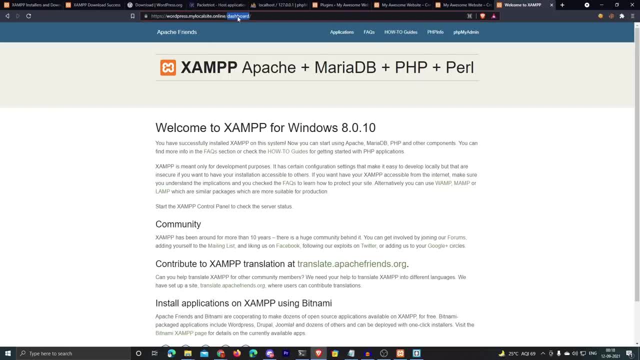 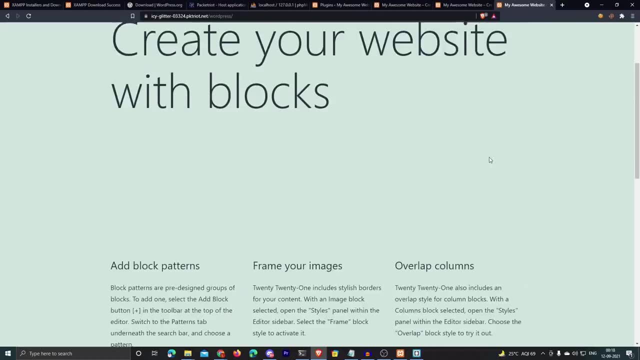 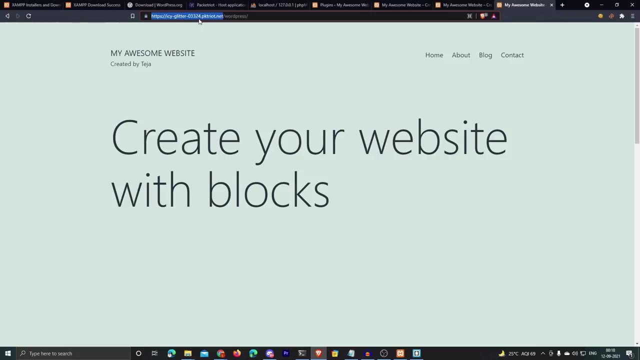 access it from our own custom domain right here. so if i just go to slash wordpress here, that is just created, um, but wait, um, there's actually one more thing you need to do. if you look at the url, it's still um pointing to our unique host name, which is not really our custom domain, which we 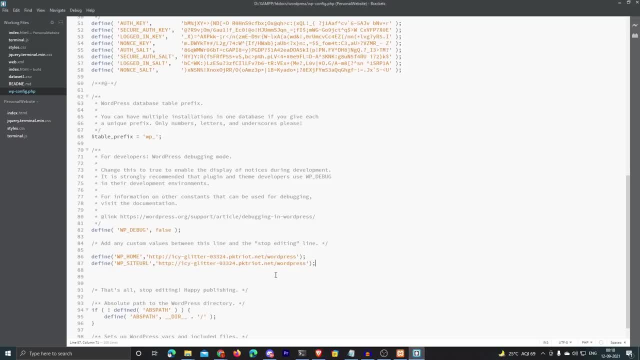 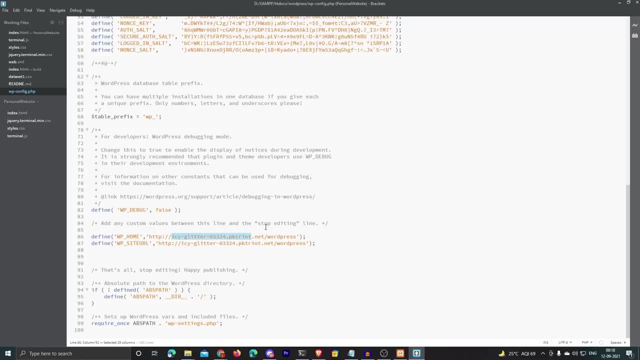 want to use this is because, um, we have to change in the wpconfig file. we have to change this to our custom domain. so just come back to your wpconfig file and change these two defined statements to your new subdomain, which is going to be wordpressmylocalsiteonline. 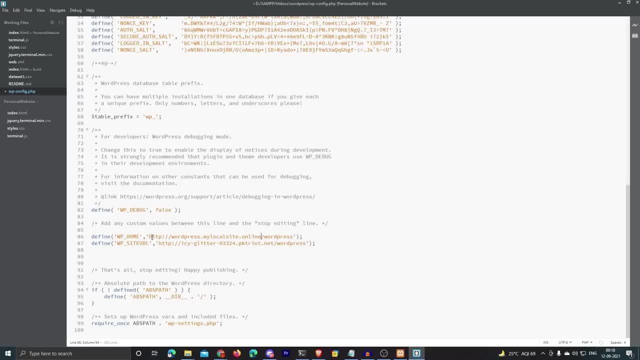 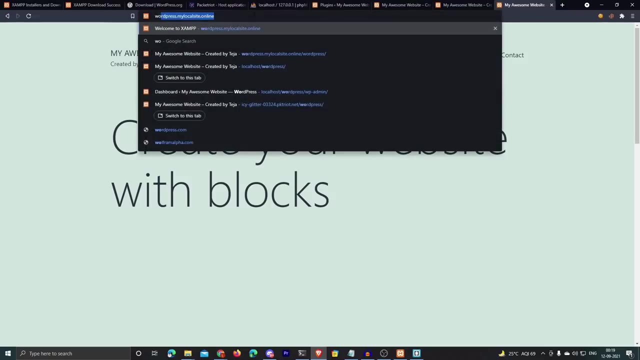 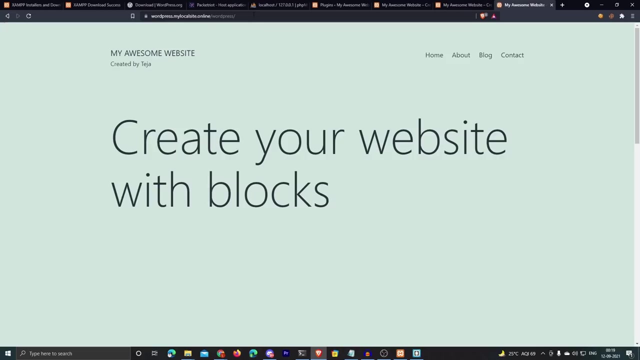 slash wordpress and i'm gonna copy the same thing for wp underscore site url as well. um, that's it. i'm just gonna save that. and now, if i go to wordpressmylocalsiteonline, slash wordpress. there you go. now you can see that we are able to access our website and you can also look. 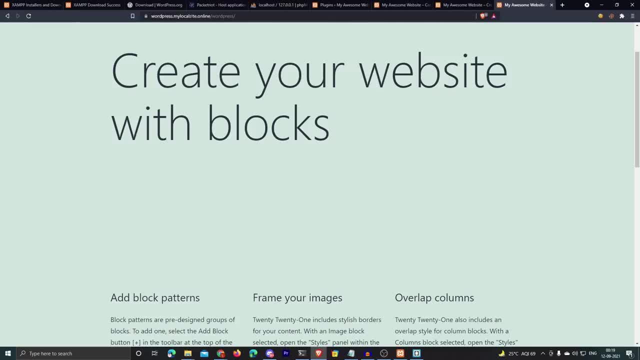 at the url. it is actually pointing to wordpressmylocalsiteonline, which is the custom domain that we are using, and you can also see that the connection is secure, which means we are using https and the certificate is encrypted. i mean, the certificate is provided by. let's encrypt.